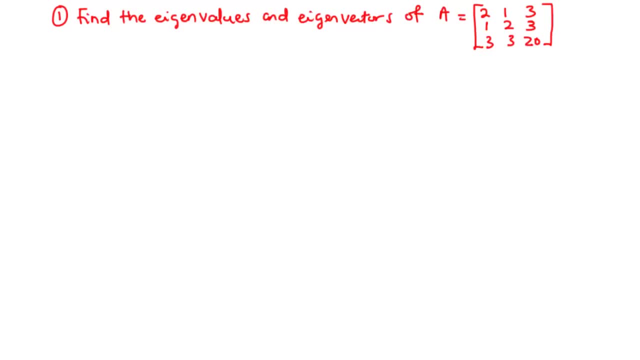 So in this video we are going to learn how to find the eigenvalues as well as the eigenvectors of a 3x3 matrix. Now let's take this example: Find the eigenvalues and eigenvectors of A. Now we have A to be a 3x3 matrix with entries 2, 1, 3, 1, 2, 3, 3, 3, 20.. 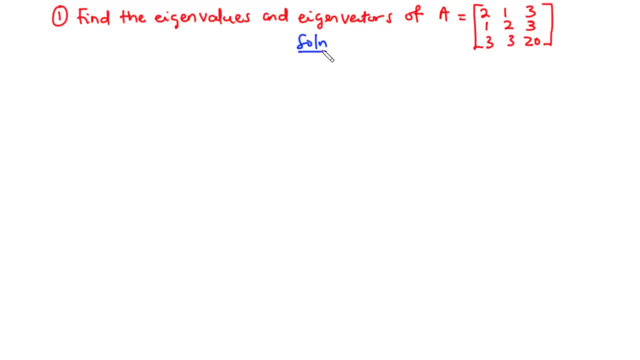 So how do we find the eigenvalues as well as the eigenvectors of matrix A? So first of all, let's find the eigenvalues. Now, the solutions to the equation given by the determinant of the matrix A minus lambda i equals zero- are the eigenvalues. So basically, we are going to use this equation to find the 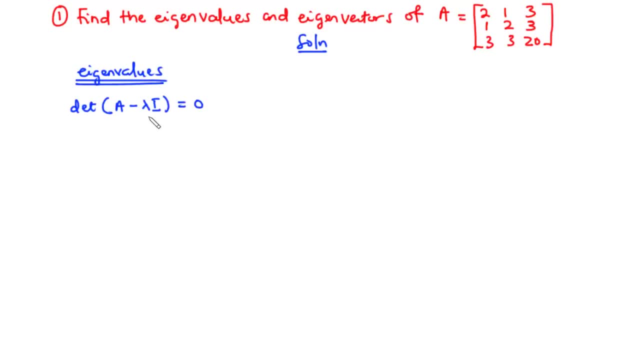 eigenvalues of matrix A. So let's try to find the matrix A minus lambda i. So A minus lambda i is equal to. we have matrix A giving us 2, 1, 3, 1, 2, 3, 3, 3, 20 minus lambda. 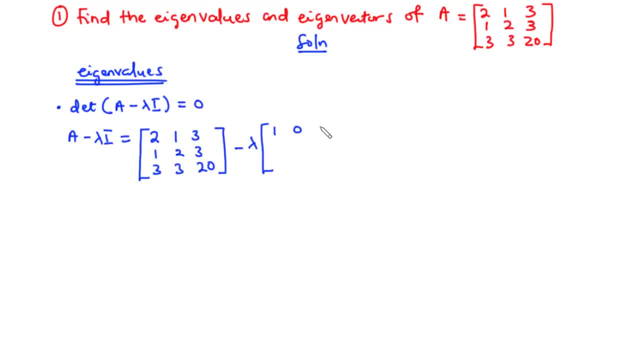 and then we have the identity matrix, which is 1, 0, 0, 0, 1, 0, 0, 0, 1.. Now let's simplify. this Lambda is going to multiply each value of the identity matrix. 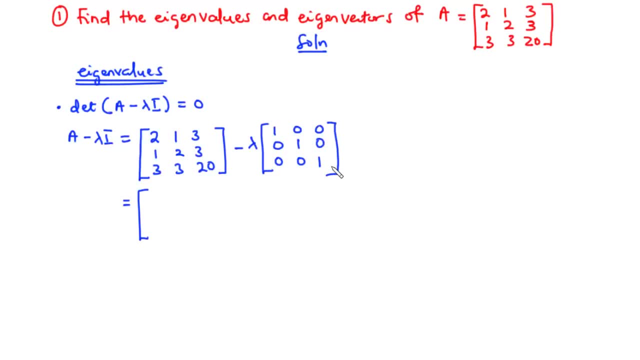 and because we have the leading diagonal containing all ones, then it means that lambda, after multiplying each of the elements here, we are going to have the element in the leading diagonal to be lambda, lambda, lambda. So basically, in simplifying this, we are going to have two minus lambda one. 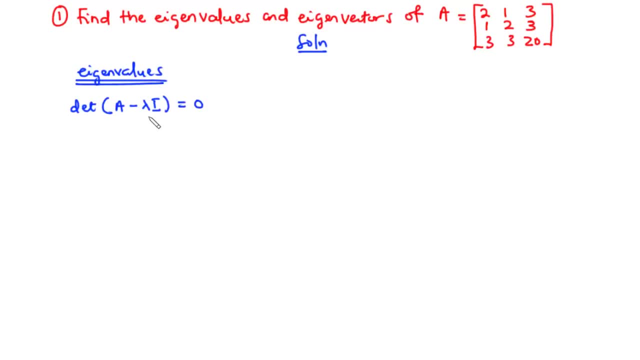 eigenvalues of matrix A. So let's try to find the matrix A minus lambda i. So A minus lambda i is equal to. we have matrix A giving us 2, 1, 3, 1, 2, 3, 3, 3, 20 minus lambda. 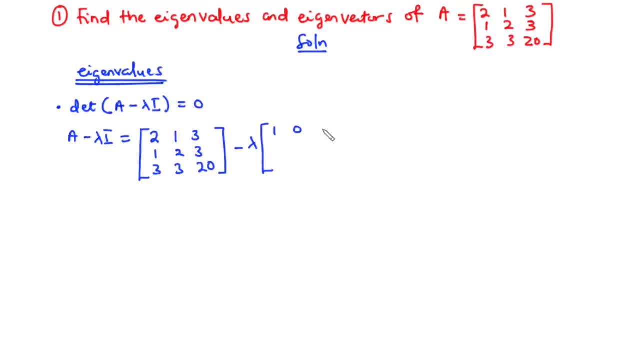 1.. And then we have the identity matrix, which is 1, 0, 0, 0, 1 0, 0, 0, 1.. Now let's simplify. this Lambda is going to multiply each value of the identity matrix and because we have the leading 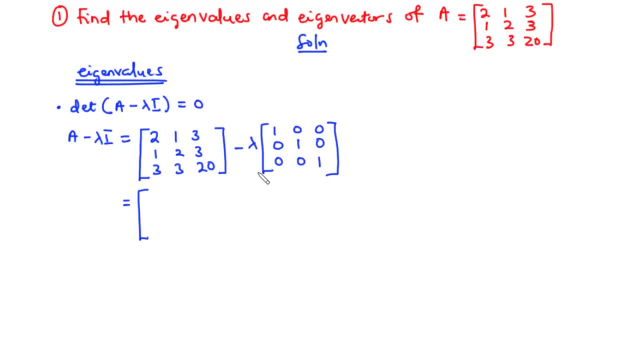 diagonal containing all ones, then it means that lambda, after multiplying each of the values, will of the elements, here we are going to have the element in the leading diagonal to be lambda, lambda, lambda. So basically, in simplifying this, we are going to have 2 minus lambda, 1, which is still 2 minus lambda. We have 1 minus 0, which is 1.. 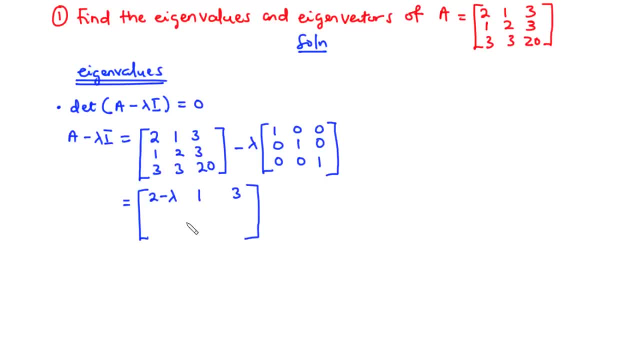 3 minus 0, which is also 3.. For row 2 we have: 1 minus 0 is 1, and then 2 minus lambda 1, which is the same as 2 minus lambda. We have 3 minus 0,, 3 minus 0,, 3 minus 0, and then 20 minus lambda 1, which is 20 minus lambda. 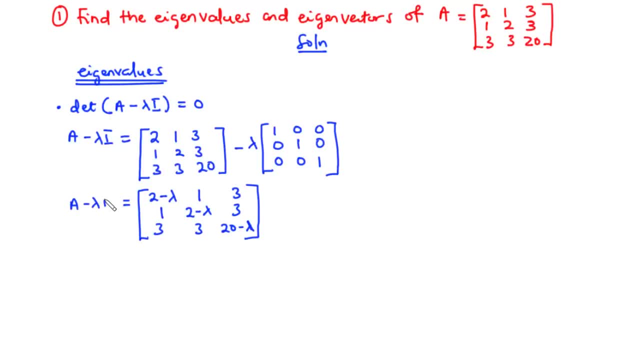 So that is the matrix A minus lambda. I Now let's find the determinant of this matrix and then equate that to 0.. So we have the determinant of the matrix containing elements: 2 minus lambda, 1, 3. 1 2 minus lambda. 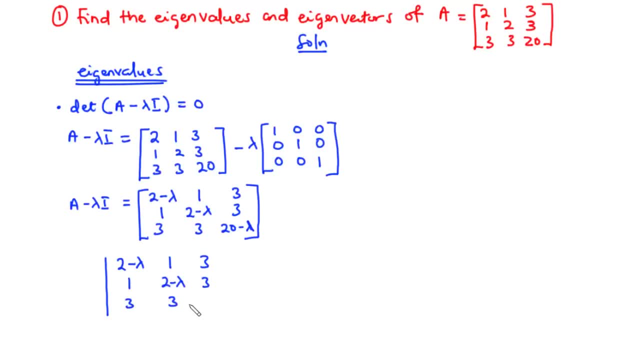 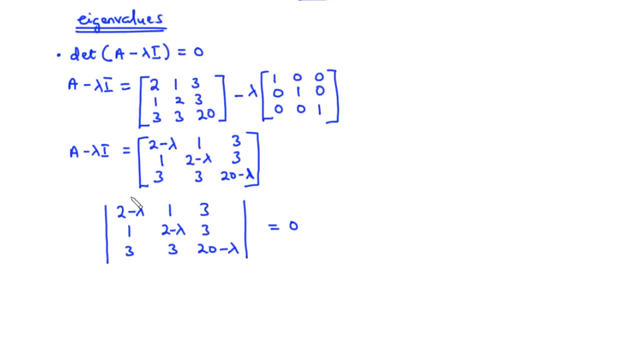 3, 3, 3, 20 minus lambda, and the determinant is equal to 0.. So let's find the determinant of this matrix. So in finding the determinant, first of all we select this value, that is, the element in row 1, column 1, and then we cancel out the. 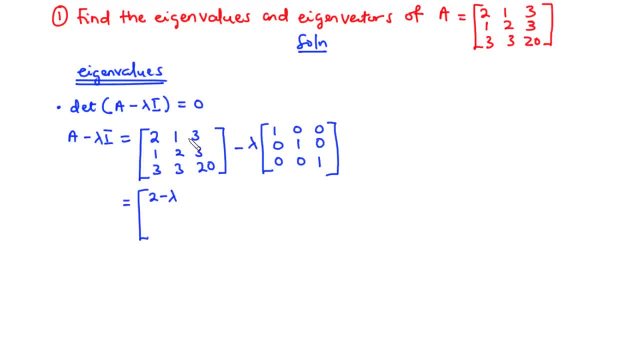 which is still two minus lambda. we have one minus zero, which is one. three minus zero, which is also three. For row two, we have: one minus zero is one, and then two minus lambda one, which is the same as two minus lambda. we have three minus zero, three minus zero. 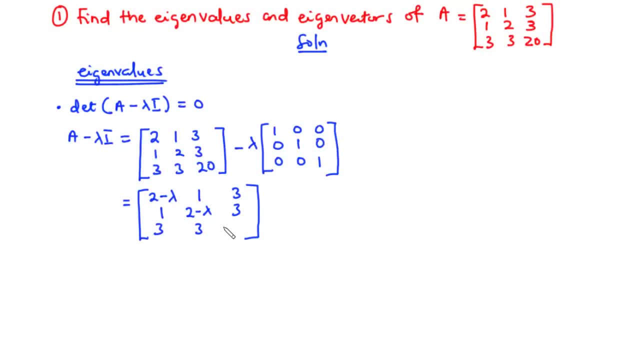 three minus zero and then 20 minus lambda, one which is 20 minus lambda. So that is the matrix A minus lambda. I. Now let's find the determinant of this matrix and then equate that to zero. So we have the determinant of the matrix containing elements: two minus lambda. 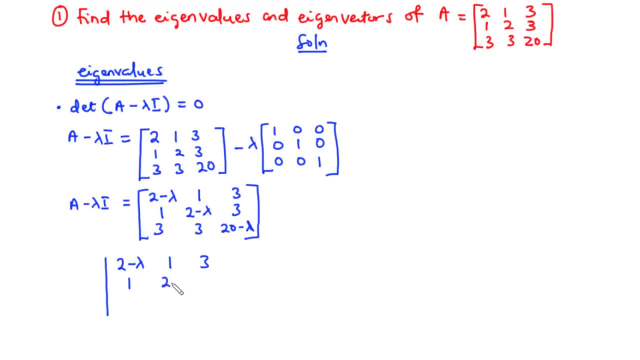 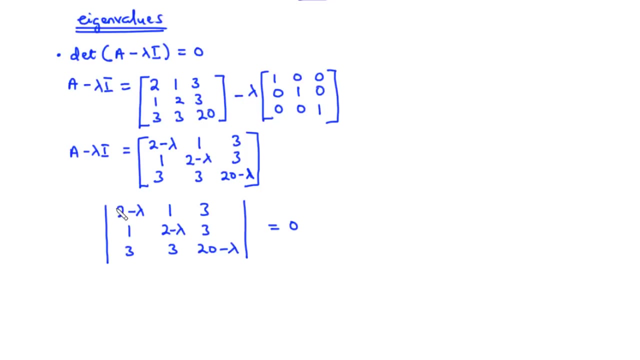 one, three, one, two minus lambda. three, three, three, 20 minus lambda, and the determinant is equal to zero, equal to 0. So let's find the determinant of this matrix. So in finding the determinant, first of all we select this value, that is the element. 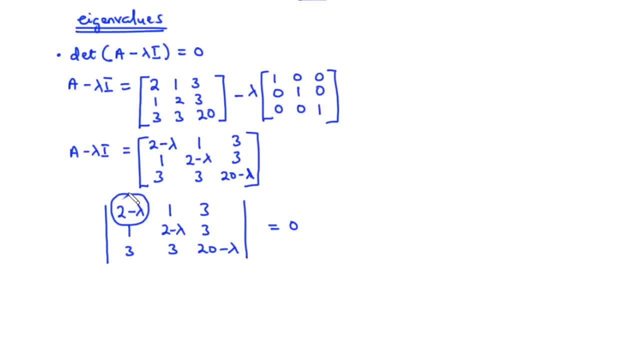 in row 1, column 1, and then we cancel out the entire row and column of this element and then we find the determinant of the resulting 2 by 2 matrix. So basically we have 2 minus lambda times. when you cancel out this row and this column, you are left with 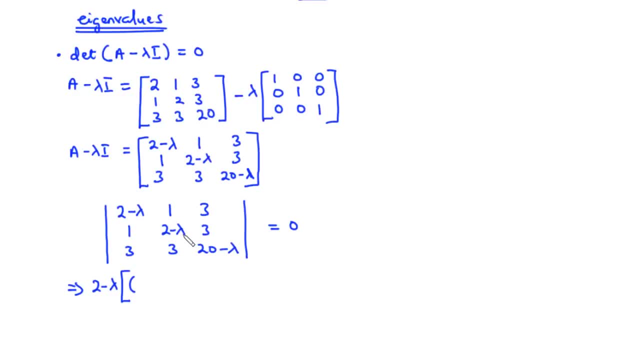 20 minus lambda times 2 minus lambda. So we have 20 minus lambda times 2 minus lambda minus 3 times 3.. And then minus. So normally it is plus minus plus. So this first value is going to be plus 2 minus lambda. Okay, And then we have: 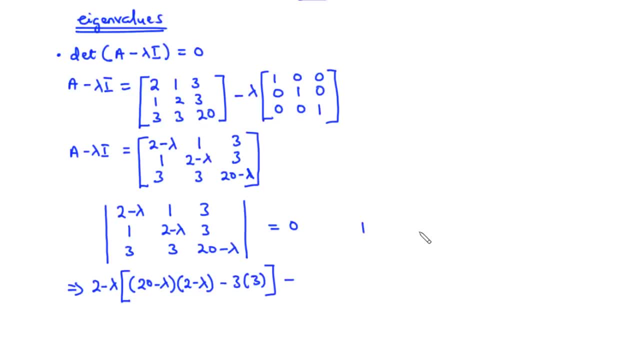 this to be minus and the next value becomes plus. So we have minus 1.. So we select this value And then we cancel out the row and column containing this value, and then we have 1,, 3,, 4, 3, 20 minus lambda. 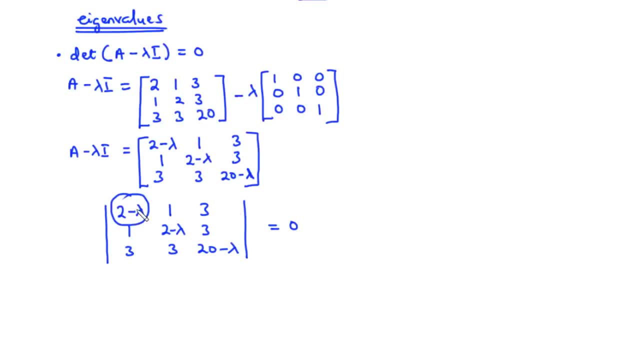 entire row and column of this element and then we find the determinant of the resulting 2x2 matrix. So basically we have 2 minus lambda times. when you cancel out this row and this column left with 20 minus lambda times 2 minus lambda. So you have 20 minus lambda times 2 minus. 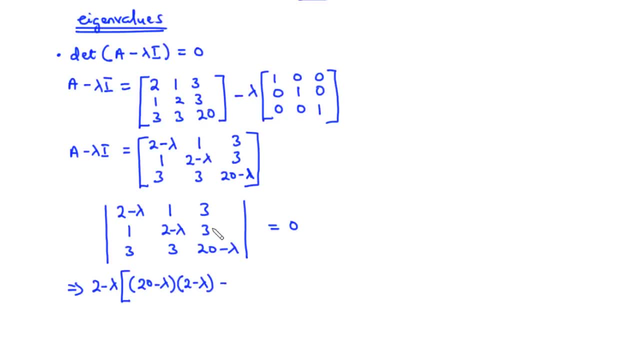 lambda minus 3 times 3.. And then minus. So normally it is plus minus plus. So this first value is going to be plus 2 minus lambda, And then we have this to be minus and the next value becomes plus, So we have minus 1.. So we select this value And then we cancel out the row and 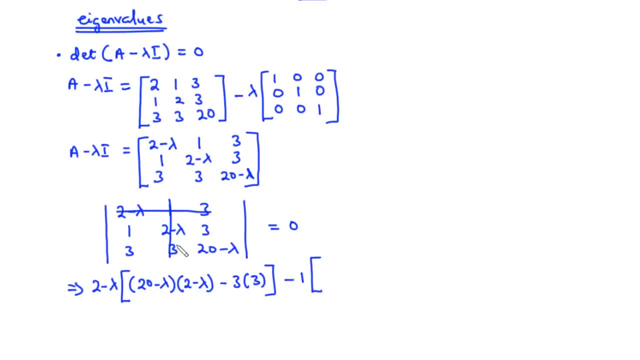 column containing this value And then we have 1,, 3,, 3,, 20 minus lambda. So we multiply 20 minus lambda by 1.. We have 20 minus lambda Times 1 minus 3 times 3. And then plus 3.. We cancel out the row and column containing 3.. 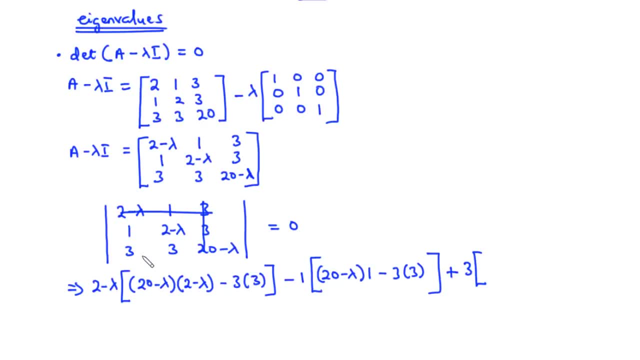 And then we have 1, 2 minus lambda, 3, 3.. So that's going to be 3 times 1 minus lambda, 2 minus 3 times 2 minus lambda, And this is equal to 0.. Now let's simplify further. So we are: 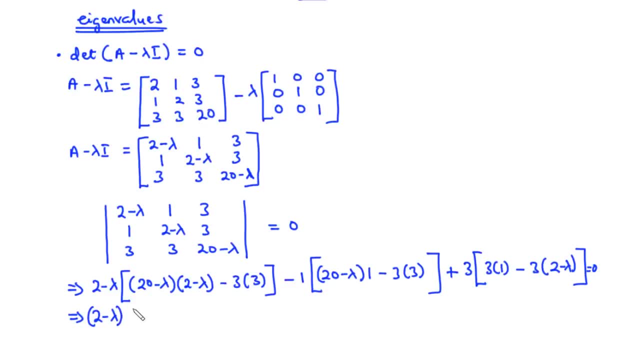 going to have 2 minus lambda. Let me put this in the bracket All times. Now we have 20 times 2, which is 40.. 20 times negative lambda: Negative: 20 lambda. 2 times negative lambda. That is negative 2 lambda And then negative lambda times negative. 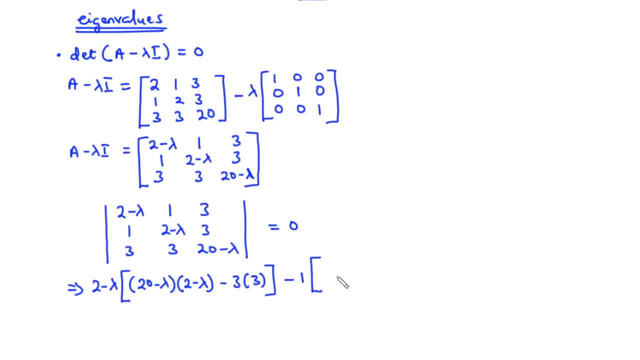 So we multiply 20 minus lambda by 1. We have 20 minus lambda times 1 minus three, times three And then plus 3.. We cancel out the row and column containing three and then we have 1, 2 minus lambda. 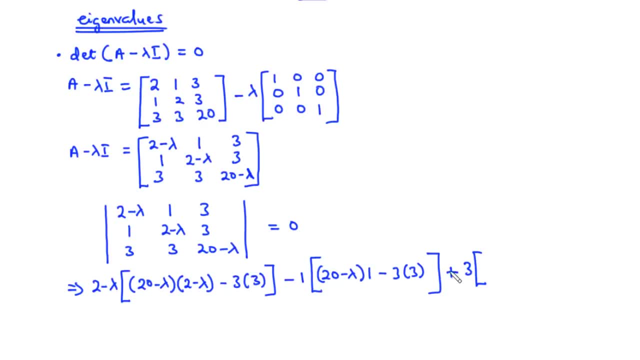 lambda 3: 3. So that's going to be 3 times 1 minus 3 times 2 minus lambda, And this is equal to 0.. Now let's simplify further. So we are going to have 2 minus lambda, let me. 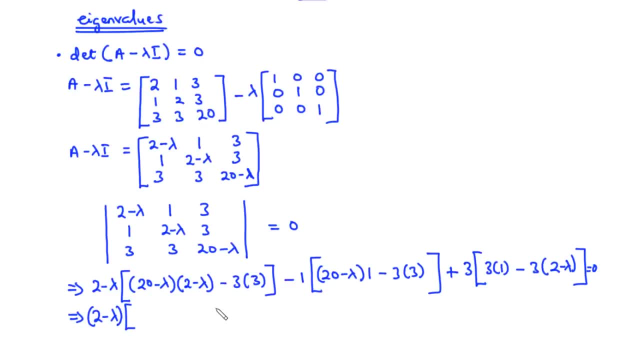 put this in the bracket all times. Now we have 20 times 2, which is 40.. 20 times negative lambda: negative 20 lambda 2 times negative lambda, that is negative 2 lambda. And then negative lambda times negative lambda, which is plus lambda square, And then we have negative. 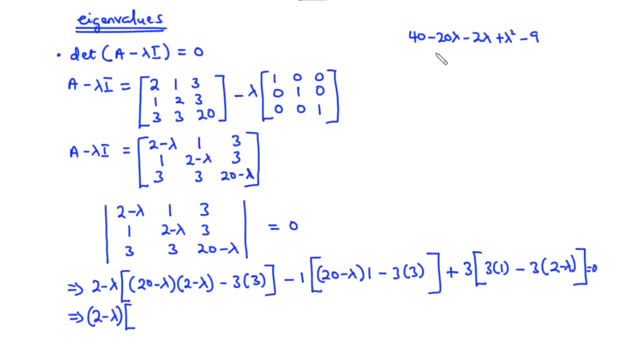 3 times 3, which is negative 9.. So we can simplify this to become lambda square minus 22, lambda, And then 40 minus 9 is 31.. So we have lambda square minus 22, lambda plus 31.. Lambda square minus 22, lambda plus 31. 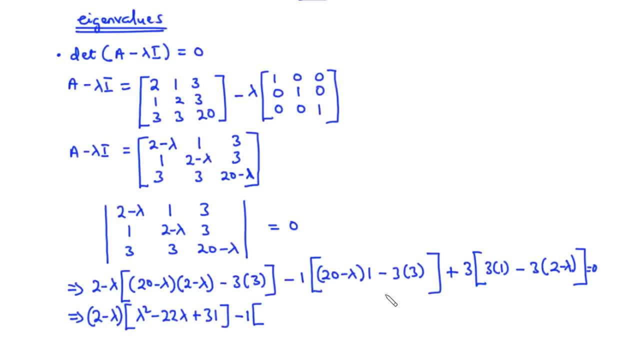 minus 1 into brackets, We have 20 minus lambda. times 1 is still 20 minus lambda. And then 3 times 3 is 9, so negative 9.. So 20 minus 9 is 11.. So we have 11 minus lambda. 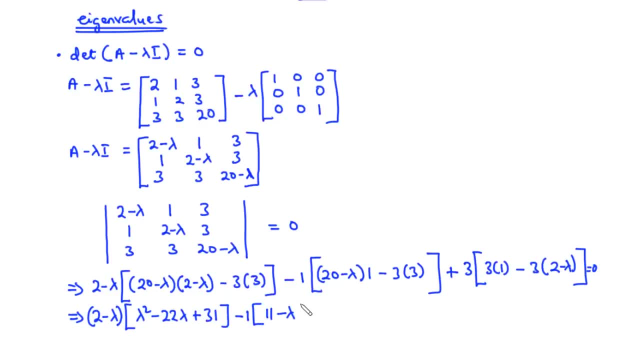 So here we have 3 times 1, which is 3. Negative 3 times 2 is negative, 6. Negative 3 times negative lambda becomes plus 3 lambda. So simplifying this, that becomes negative 3 plus 3 lambda. 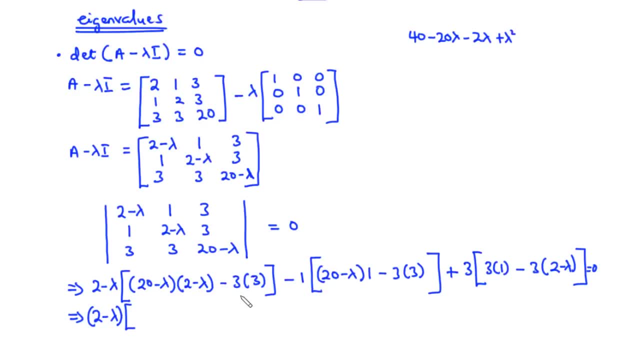 lambda, which is plus lambda square, And then we have negative 3 times 3,, which is negative 9.. So we can simplify this to become lambda square minus 22 lambda, And then 40 minus 9 is 31.. So we have lambda square minus 22, lambda plus 31.. 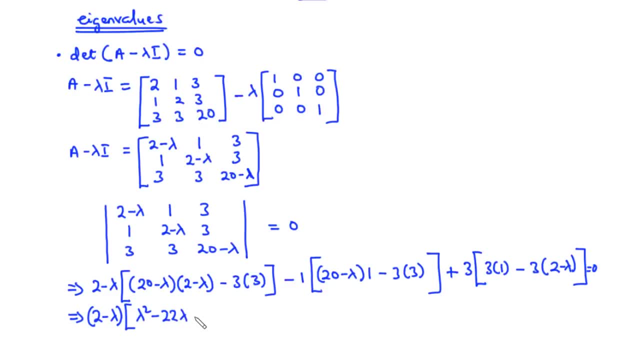 Lambda square minus 22 lambda plus 31 minus 1 into brackets We have 20 minus lambda. times 1 is still 20 minus lambda. And then 3 times 3 is 9.. So negative 9.. So 20 minus 9 is 11.. So we have 11 minus lambda. 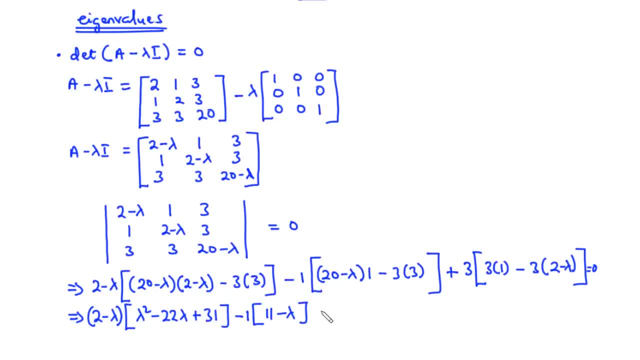 OK, So here we have 3 times 1, which is 3. Negative 3 times 2 is negative, 6. Negative 3 times negative lambda becomes plus 3 lambda. So simplifying this, that becomes negati спасибо-3. 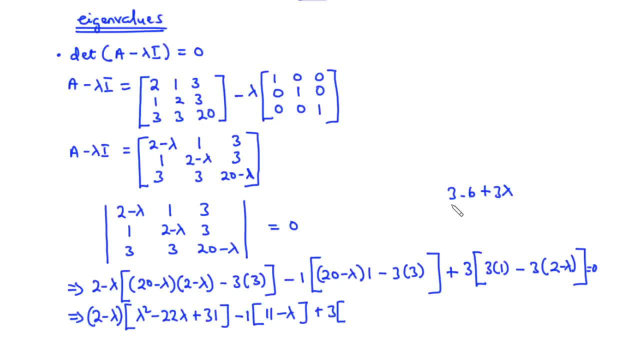 oraxal: 2의x plus 3 lambda, So negative 3 plus 3 lambda. Let's further simplify this. So we are going to multiply 2 and the negative lambda across, So we have 2 times lambda square, which gives: 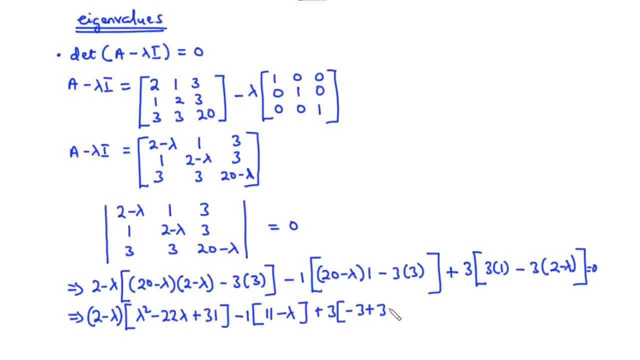 So negative 3 times 2 is negative 6.. Negative 3 times negative lambda becomes plus 3 lambda. Let's further simplify this. So we are going to multiply 2 and the negative lambda across, So we have 2 times lambda squared, which gives 2 lambda squared. 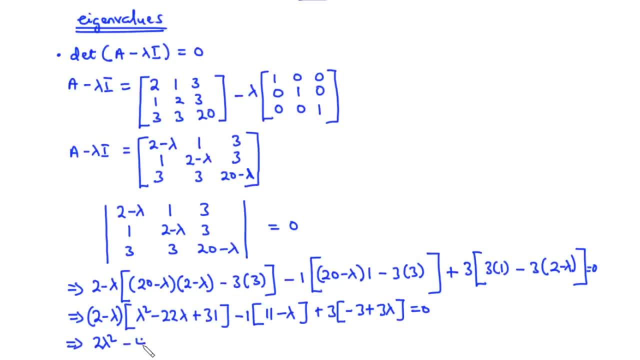 2 times negative: 22 lambda. that becomes negative 44 lambda 2 times 31,. that is 62.. Now negative lambda times lambda squared is negative lambda cubed. Negative lambda times negative: 22 lambda. that becomes plus 22 lambda squared. 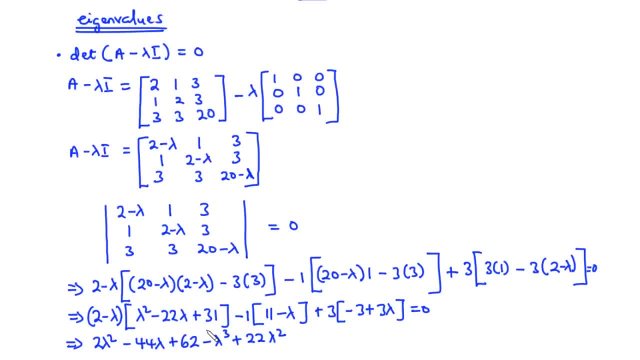 And then negative lambda times 31 becomes negative 31 lambda. Negative 1 times 11 becomes negative 11.. Negative 1 times negative lambda becomes plus lambda. 3 times negative 3, that is negative 9.. And then 3 times 3 lambda becomes 9 lambda. 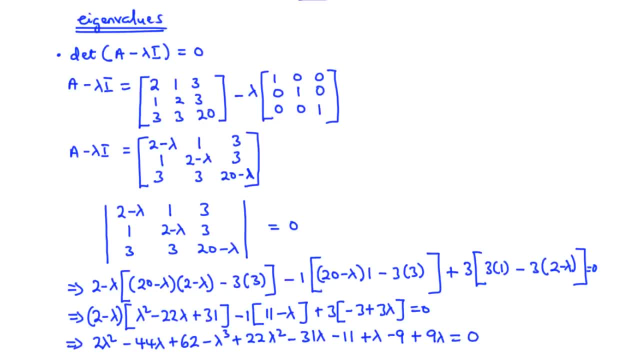 And we have this all equals 0.. Let's further simplify. So here we have negative lambda cubed. We have 2 lambda squared plus 22 lambda squared, And that gives plus 24 lambda squared. Now for values of lambda. we have negative 44 minus 31.. 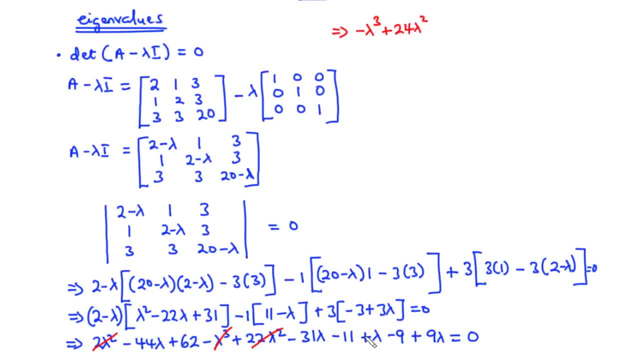 And that becomes negative 75 plus lambda, That becomes negative 74, and then plus 9 lambda, And that becomes negative 65. So we have negative 65. And that becomes negative 64. And that becomes negative 75 lambda. Now for the constants, we have 62 minus 11, minus 9.. 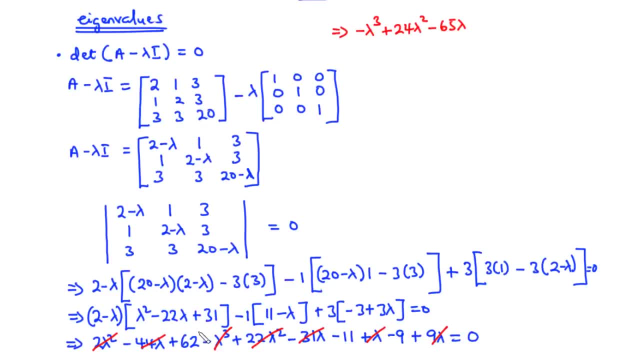 Now negative 11 minus 9 is negative 20.. Therefore, 62 minus 20 is 42.. Now let's multiply each term of the equation by negative 1.. So that's the equation. So the equation becomes: lambda cubed minus 24. lambda squared plus 65. lambda minus 42 equals 0.. 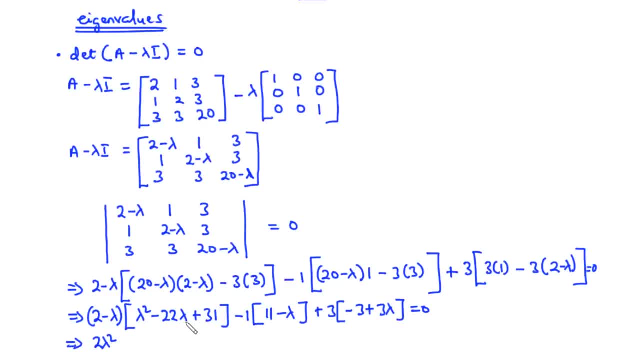 2 lambda square 2 times negative. 22 lambda, That becomes negative, 44 lambda 2 times 31.. That is 62.. Now negative lambda times lambda square is negative lambda cube. Negative lambda times negative. 22 lambda, That becomes plus 22 lambda square And then negative lambda. 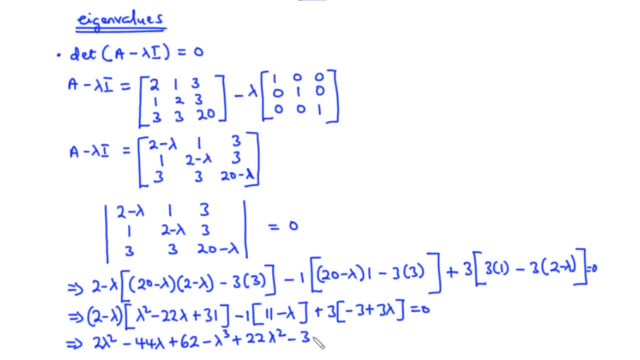 times 31 becomes negative 31 lambda. Negative 1 times 11 becomes negative 11.. Negative 1 times negative lambda becomes plus lambda, 3 times negative 3. That is negative 9. And then 3 times 3 lambda becomes 9 lambda And we have this: all equals 0.. Let's further simplify. 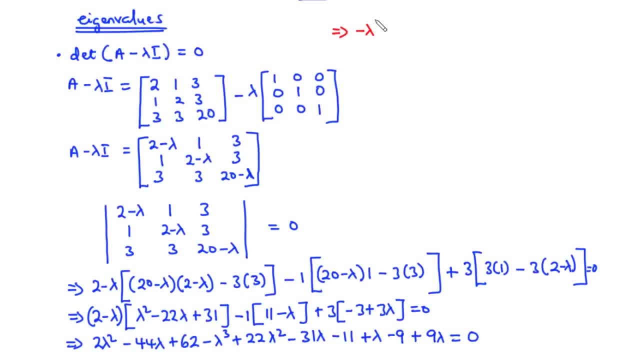 So here we have negative lambda cube. We have 2 lambda square plus 22 lambda square, And that gives plus 24 lambda square. Now for values of lambda, we have negative 44 minus 31. And that becomes negative 75.. 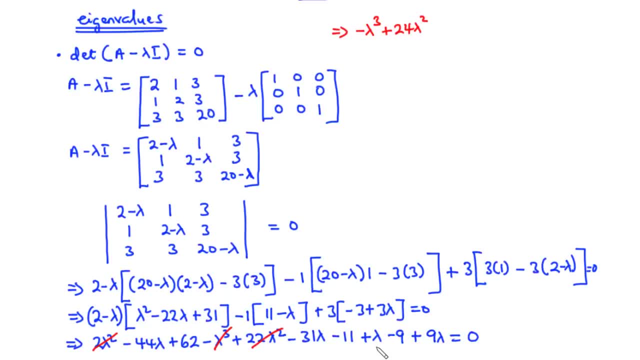 Plus lambda, That becomes negative 74. And then plus 9 lambda And that becomes negative 65. So we have negative 65 lambda. Now for the constants, we have 62 minus 11 minus 9.. Now negative: 11 minus 9 is negative 20.. Therefore, 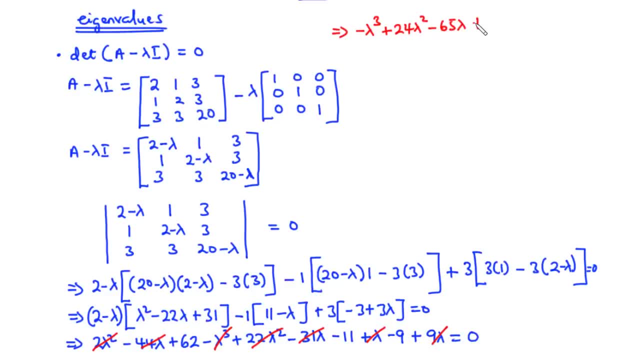 62 minus 20.. is 42.. Now let's multiply each term of the equation by negative one, so that the equation becomes lambda cubed minus 24. lambda squared plus 65. lambda minus 42 equals 0.. So here we have a cubic equation and therefore we are going to 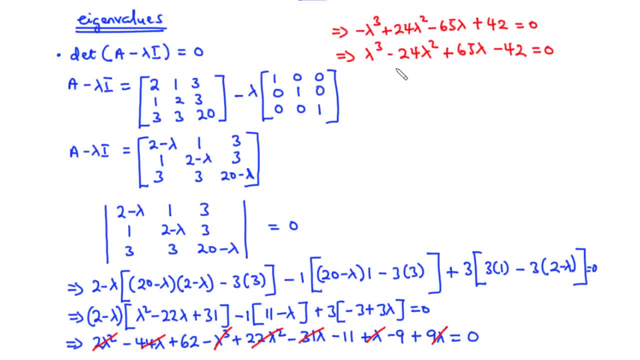 obtain three values of lambda. So at this point we can test values of lambda that will make this whole equation go to zero. So you can basically test values like lambda equals 1. lambda equals negative 1. lambda equals 2. lambda equals negative 2.. 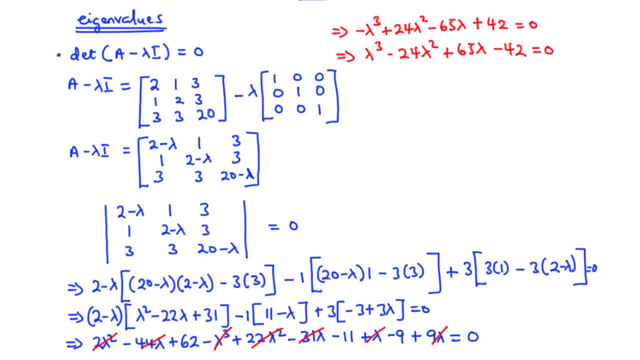 Now, for the sake of time, if you should punch this on your calculator, on your scientific calculator, then you are going to have values of lambda to be: lambda equals 1, lambda equals 2. lambda equals 21.. So these are the roots of the equation and these are the 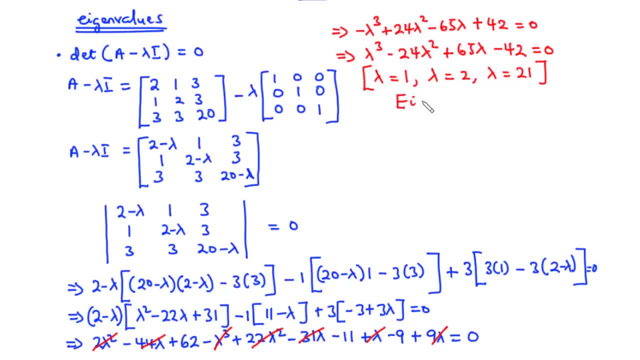 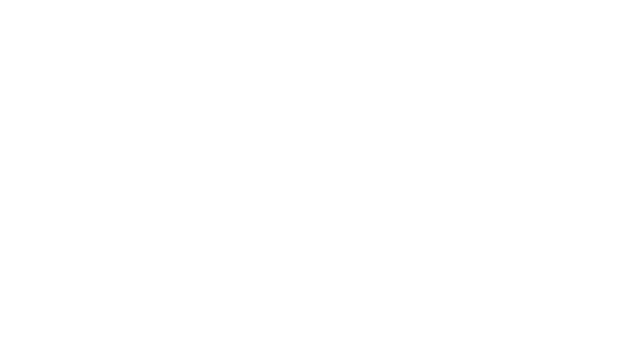 eigenvalues of A. So once we have the eigenvalues of A, then we are going to find the eigenvector that corresponds to each of the eigenvalues. So that is what we are going to do in our next step. So in finding the eigenvectors that corresponds to each eigen value, first of 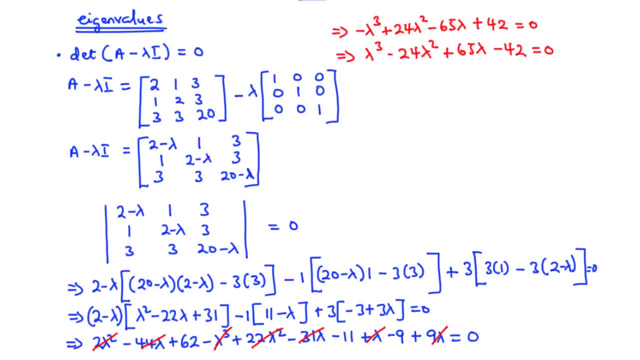 So here we have a cubic equation And therefore we are going to obtain 3 values of lambda. So at this point we can test values of lambda that will make this whole equation go to 0. So we can basically test values like lambda. 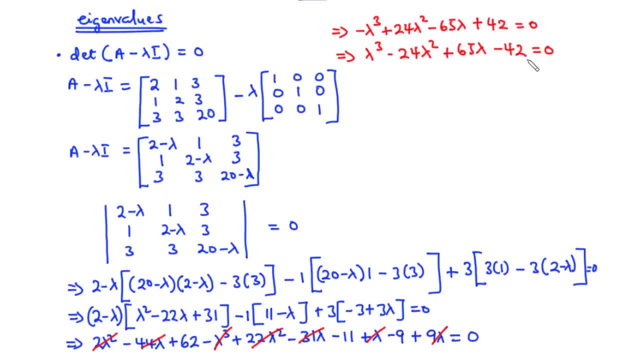 lambda equals 1, lambda equals negative 1, lambda equals 2, lambda equals negative 2.. And now, for the sake of time, if you should point this on your calculator, on your scientific calculator, then you are going to have values of lambda to be: lambda equals 1, lambda equals. 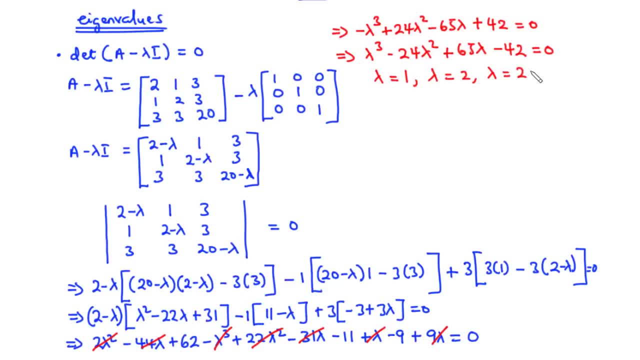 2 lambda equals 21.. So these are the roots of the equation And these are the eigenvalues of A, So let me just write it down. So, whatever the root of the equation, multiple times 1.. 2. lambda equals 1.. 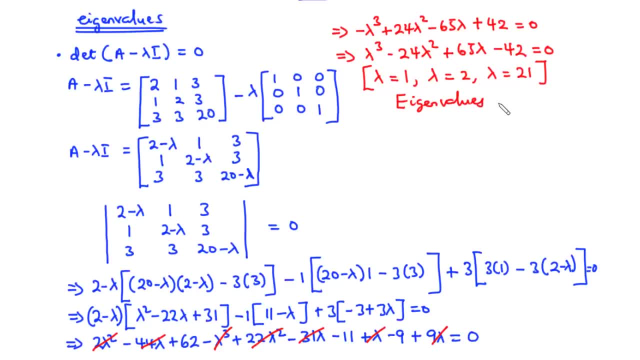 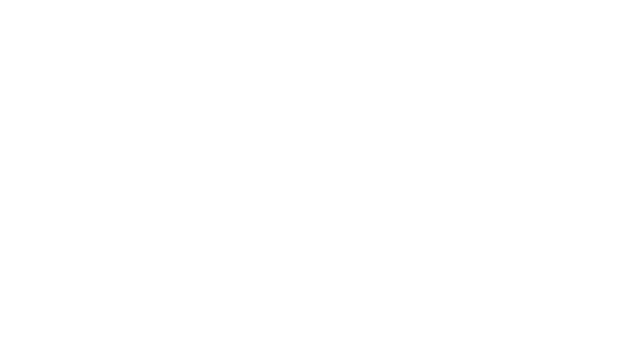 2. So once we have the eigenvalues of A, then we are going to find the eigenvector that corresponds to each of the eigenvalues. So that is what we are going to do in our next step. So in finding the eigenvectors that corresponds to each eigenvalue, first of all, let's assume 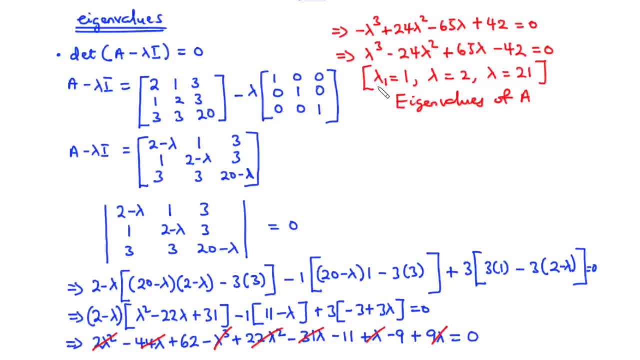 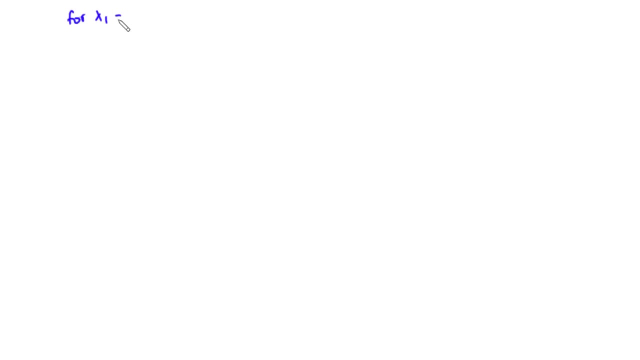 that we have lambda1 to be equal to 1, lambda2 equals 2 and then lambda3 equals 21.. So for lambda1 equals 1, we are going to find the eigenvector that corresponds to lambda1 equals 1.. 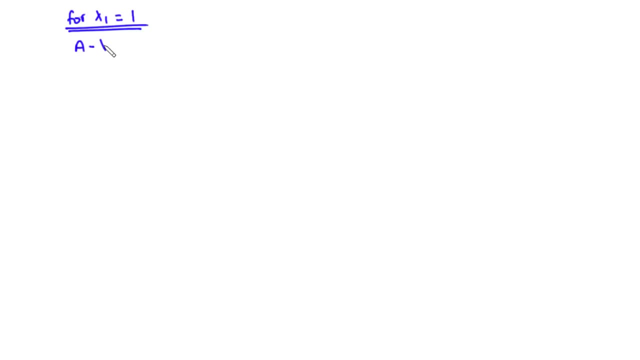 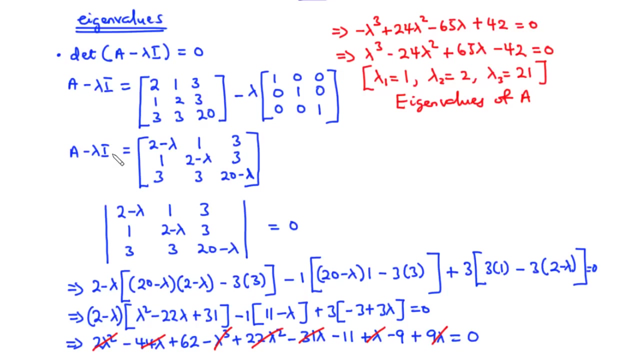 Now using the equation A minus lambda i, all times x equals 0 or, better still, the 0 vector. We already solved for A minus lambda i. that is the matrix A minus lambda i. So let's go back and then write that: So this is the matrix A minus lambda i, and that is giving us. 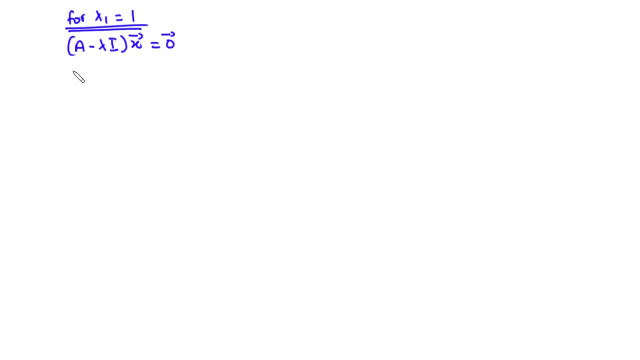 2 minus lambda, 2, 1, 3, 1, 2 minus lambda, 3, 3, 3, 20 minus lambda. So that is a minus lambda i. Then we are going to multiply this whole thing by the eigenvector, which has components x1. 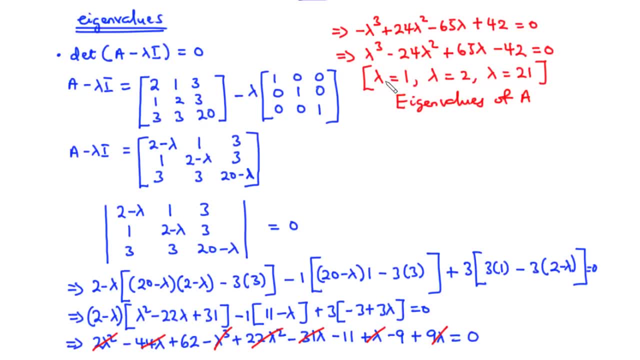 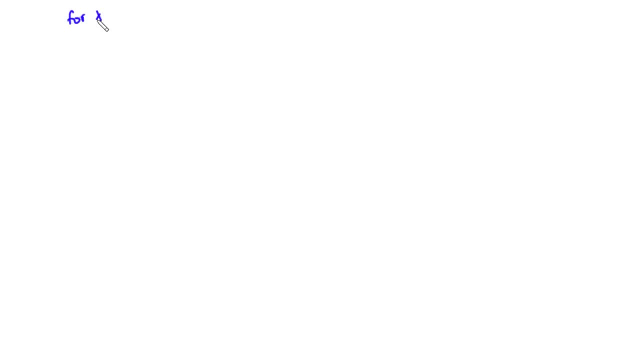 all. let's assume that we have lambda 1 to be equal to 1, lambda 2 equals 2 and then lambda 3 equals 21.. So for lambda 1 equals 1, we are going to find the eigenvector that corresponds to lambda 2.. 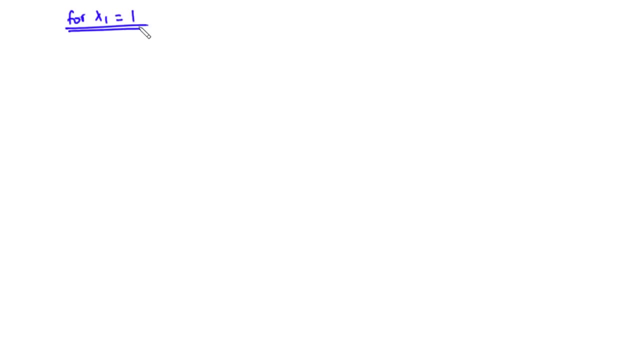 find the eigenvector that corresponds to lambda 1 equals 1.. Now, using the equation a minus lambda i, all times x equals 0, or better still, the 0 vector We already solved for a minus lambda i. that is the matrix a minus lambda i. So let's go back and then write that. 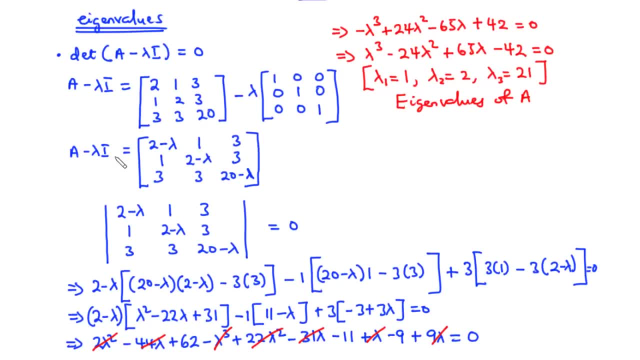 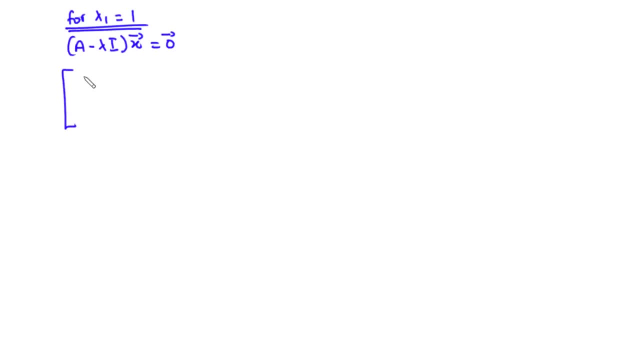 So this is the matrix a minus lambda i, and that is giving us 2 minus lambda, 1, 3, 1. 2 minus lambda, 3, 3, 3, 20 minus lambda. So that is a minus lambda i, and then we have a minus lambda i. 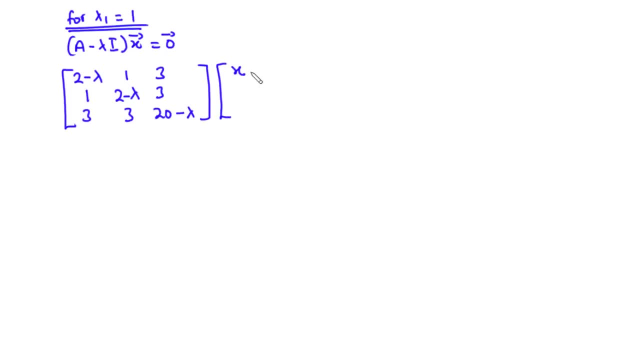 And we are going to multiply this whole thing by the eigenvector, which has components x1, x2, x3 equals the 0 vector having components 0, 0, 0. Now, since we have the value of lambda, or, better still, the value of lambda 1 equals 1, we are going to substitute that here. 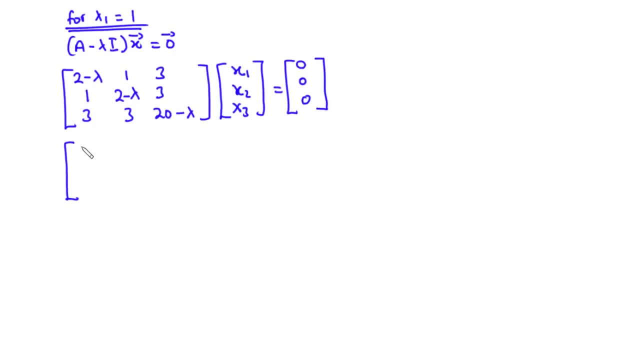 So if lambda is equal to 1, then we have 2 minus 1.. Which is 1.. We have 1, 3, 1. 2 minus 1 is 1, 3, 3, 3, 20 minus 1 is 19.. 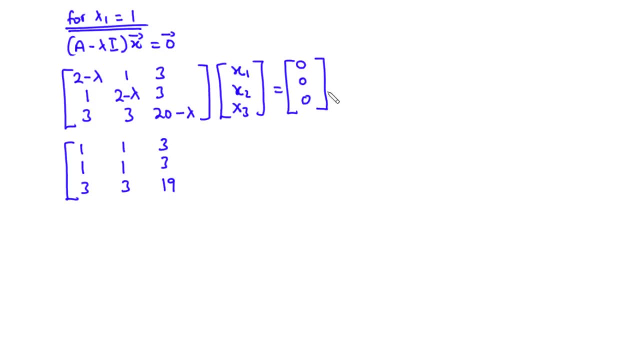 Now, at this point, we are going to convert this system of equations into an augmented matrix. So, after writing down the matrix a minus lambda i, We are going to have on the right hand side 0, 0, 0, which are the values on the right hand side of the equal to sign. 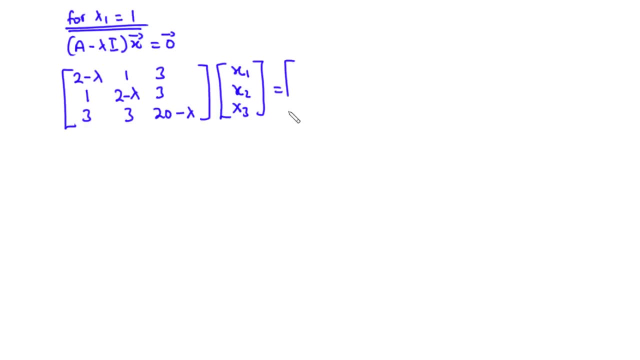 x2. x3 equals the zero vector, Of course having components 0- 0- 0.. Now, since we have the value of lambda, or better still, the value of lambda 1 equals 1, we are going to substitute that here. So if lambda is equal to 1, then we have 2. 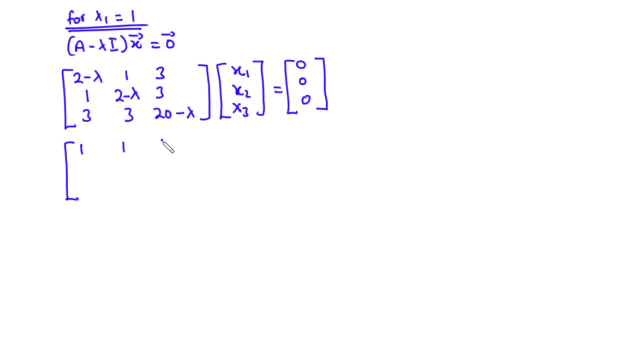 minus 1, which is 1, we have 1, 3, 1. 2 minus 1 is 1, 3, 3, 3. 20 minus 1 is 19.. Now, at this point, we are going to convert this system of equations into an augmented matrix. So, after writing down the matrix, 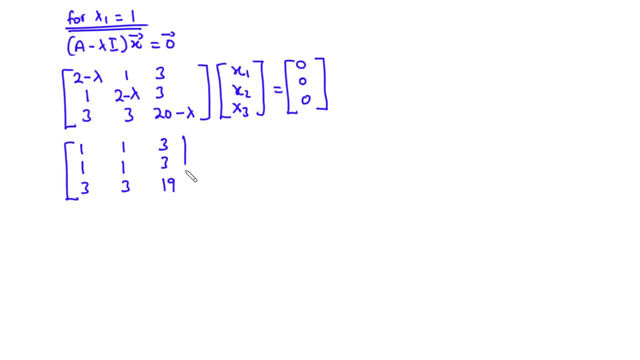 a minus lambda i. we are going to have 1, the right hand side, 0, 0, 0, which are the values on the right hand side of the equal to sign. Now we are going to perform elementary row operations on this matrix to convert this: 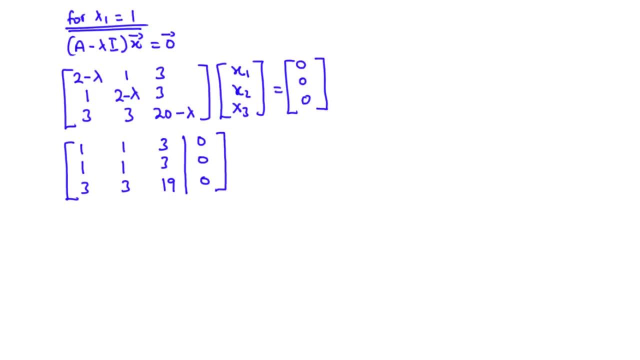 matrix to the row echelon form, so that we can find the values of x1, x2, x3, hence the eigenvector that corresponds to lambda 1.. So that is exactly what you are going to do Now: we are going to make this element and this element go to 0.. So what do we do? We are going to apply the operation. 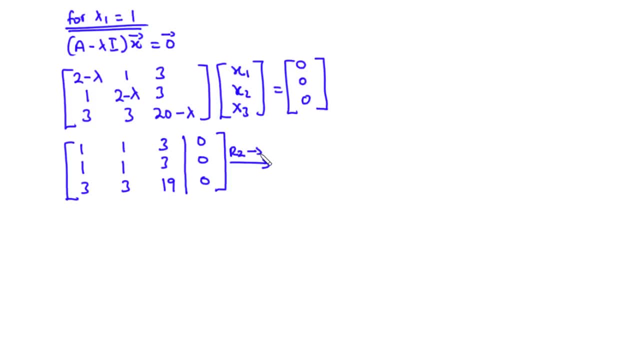 on row 2, and the operation is: we are going to subtract row 1 from row 2.. So that's going to be r2 minus r1, and then for row 3, we are going to multiply row 1 by r2 minus r1.. So that's going to be r2 minus r1.. 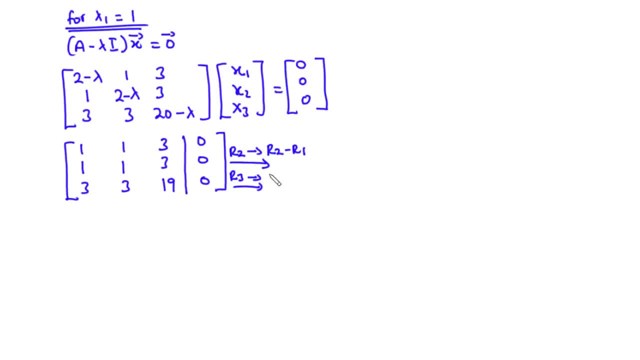 by three and then subtract that from row three, so that is row three minus three times of row one. so let's do that, so element in row one remains the same. now to row two. we have one minus one, which is zero. one minus one is zero. three minus three is zero. 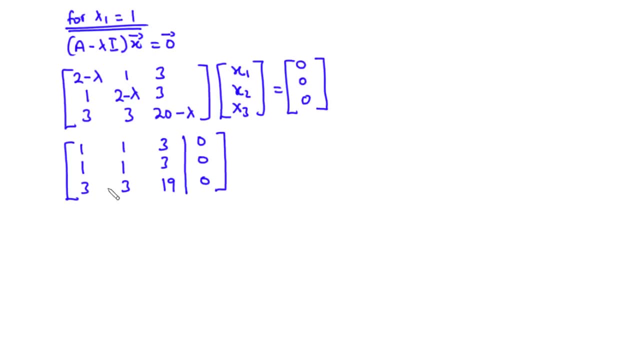 Now we are going to perform elementary row operations on this matrix, to convert this matrix to the row echelon form, so that we can find the values of x1, x2, x3, hence the eigenvector that corresponds to lambda 1.. So that is exactly what you are going to do. Now we are going. 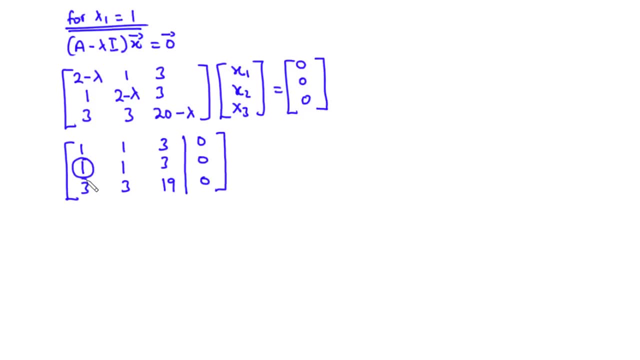 to make This element and this element Go to 0.. So what we do, We are going to apply the operation on row 2.. And the operation is: We are going to subtract row 1 from row 2.. So that is going to be R2 minus R1.. 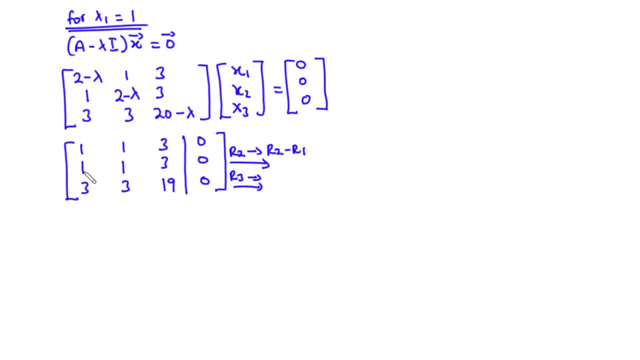 And then for row 3.. We are going to multiply Row 1 by 3.. and then subtract that from row three, So that is row three minus three times of row one. So let's do that. So elements in row one remains the same. 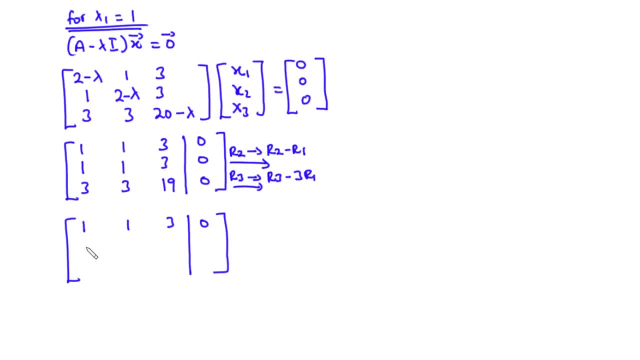 Now to row two. we have one minus one, which is zero. one minus one is zero. three minus three is zero. and then zero minus zero is zero. For row three, we have three minus three times one. So three minus three is zero. Three minus three times one, that is also zero. 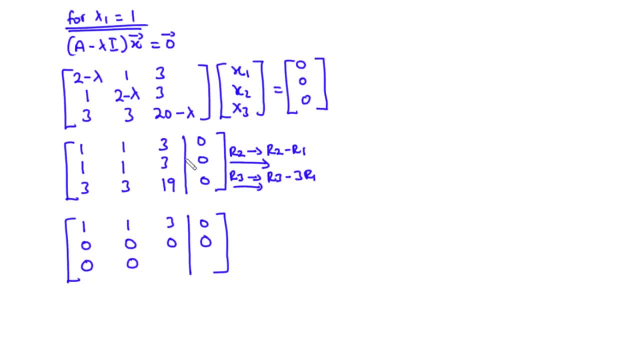 We have nineteen minus three times three. Now, three times three is nine. Nineteen minus nine is ten, And then zero minus three times zero is also zero. Next, since we have row two containing all zeros, we are going to interchange row two. 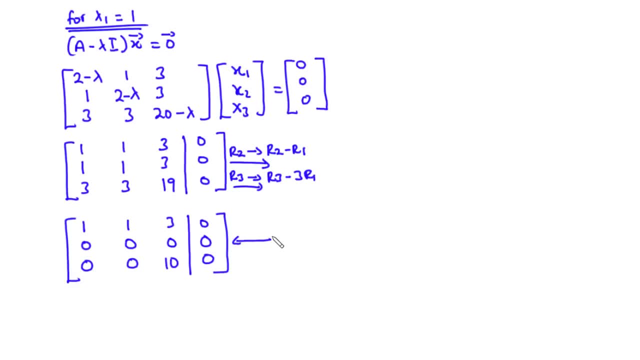 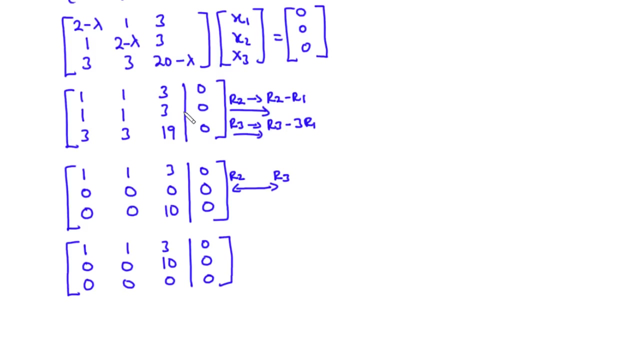 and then row three. So we interchange row two and row three, So that we have one, one, three, zero, zero, zero, ten, zero, and then zero, zero, zero, zero. So this is the row echelon form of this augmented matrix. 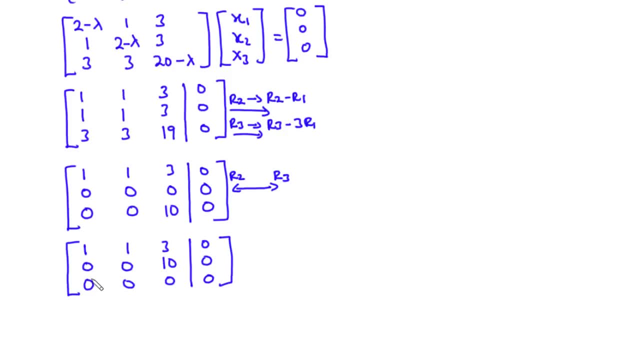 Now, focusing on row three, you realize that we have zero, zero. zero equals zero. Column one corresponds to values of x1.. Column two, values of x2, and then column three, values of x3. So that's going to be zero, x1 plus zero, x2 plus zero, x3 equals zero. 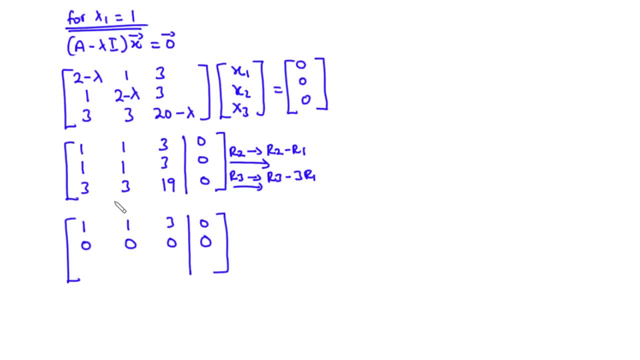 and then zero minus zero is zero for three. we have three minus three times one. so three minus three is zero. three minus three times one, that is also zero. we have nineteen minus three times three. now, three times three is nine. nineteen minus nine is ten, and then zero minus three times zero. 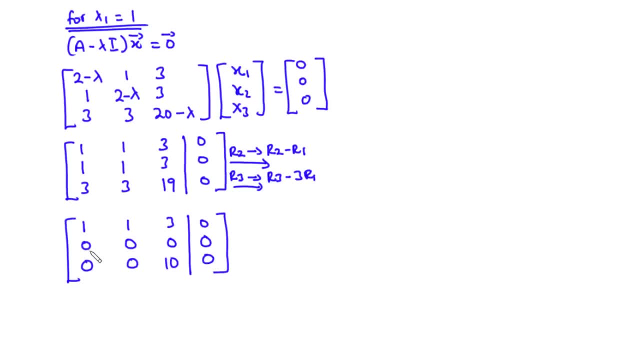 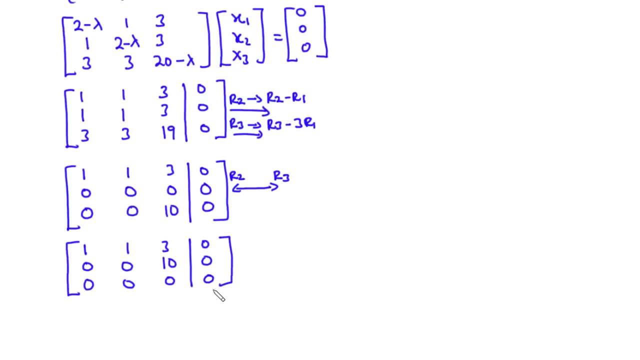 is also zero next. so, since we have row two containing all zeros, we are going to interchange row two and then row three. so we interchange row two and row three so that we have one, one, three, zero, zero, zero, ten, zero and then zero, zero, zero, zero. so this is the row echelon form of this augmented matrix. now, focusing on row three, you realize that 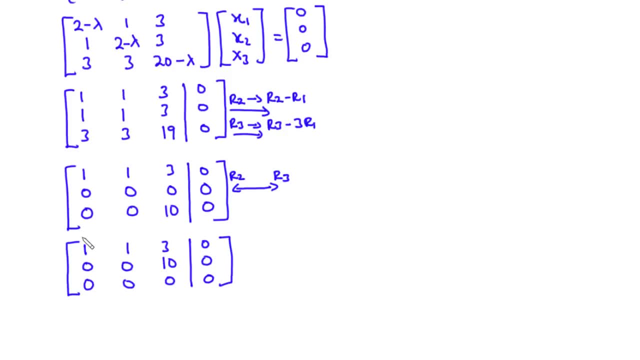 we have zero, zero. zero equals zero. column one corresponds to values of x1, column two values of x2 and then column three values of x3, so that's going to be 0x1 plus 0x2 plus 0x3 equals zero. 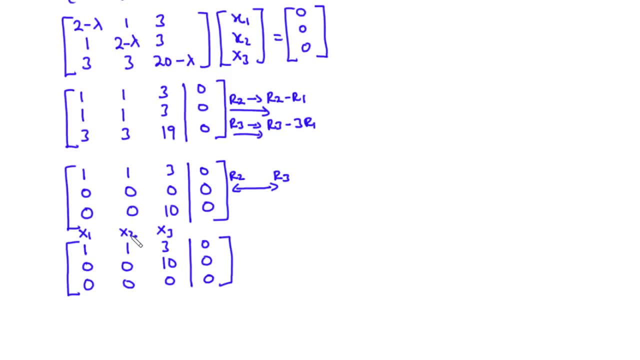 now let's move on to row 2. so that's going to be 10 x3 equals 0. so if you have 10 x3 equals 0, then definitely we know that if you divide through by 10, you have x3 equals 0, because 0 divided by 10 is still 0. 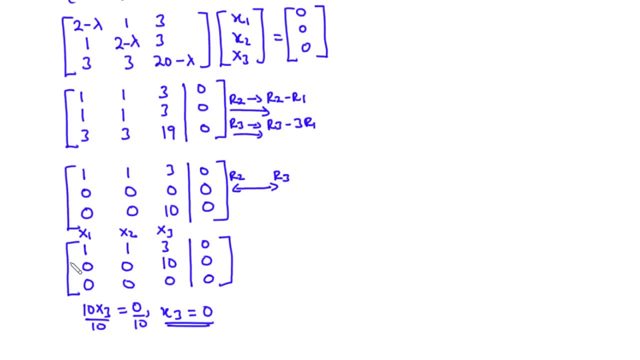 so we have the value of x3 to be 0. now, focusing on row 1, we are going to have x1 plus x2 plus 0 equals 0, so we can simplify this as x1 plus x2 equals 0. now we can transpose x2 to the right hand side so that becomes negative x2. 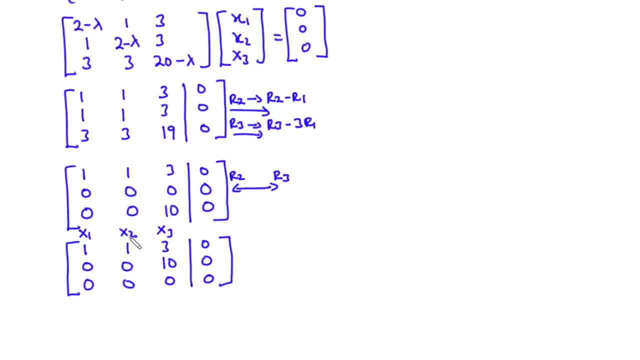 Now let's move on to row two. So that's going to be: ten x3 equals zero. So if you have ten x3 equals zero, then definitely we know that if you divide three by ten, you have x3 equals zero, because zero divided by ten is still zero. 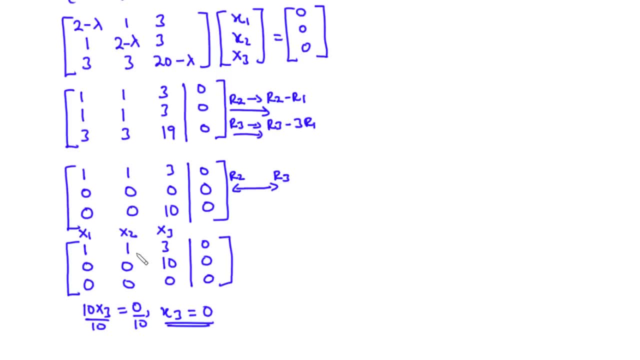 So we have the value of x3 to be zero. Now, focusing on row one, we are going to have: x1 plus x2 plus zero equals zero, So we can simplify this as x1 plus x2 equals zero. Now we can transpose x2 to the right hand side so that becomes negative x2.. 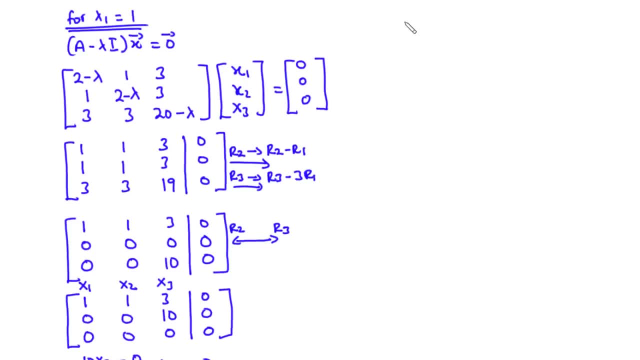 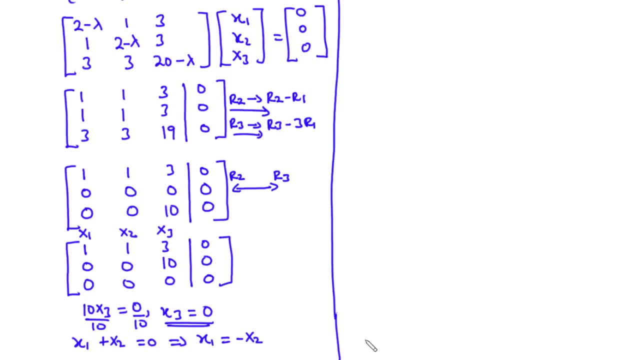 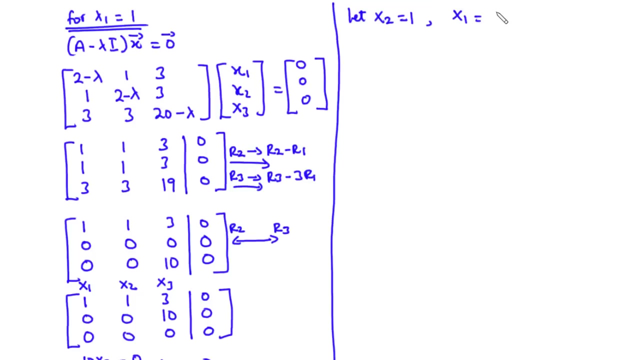 And then at this point we are going to choose any arbitrary value for x2.. So we can say that let x2 equals one. Now, if x2 equals one, then x1 becomes negative one. So we have x1 equals negative one. Therefore, the eigenvector X, which has components x1, x2, x3,, 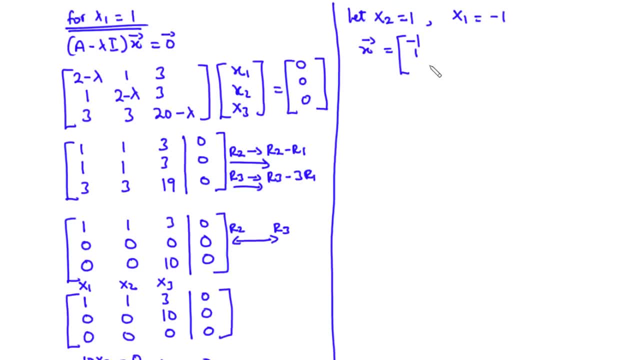 becomes negative one. 1: 0 is the eigenvector of a. that corresponds to the eigenvalue lambda 1 equals 1. now let's move on to the second eigenvalue, that is for: lambda 2 equals 2. now, if lambda 2 is equal to 2 or for: 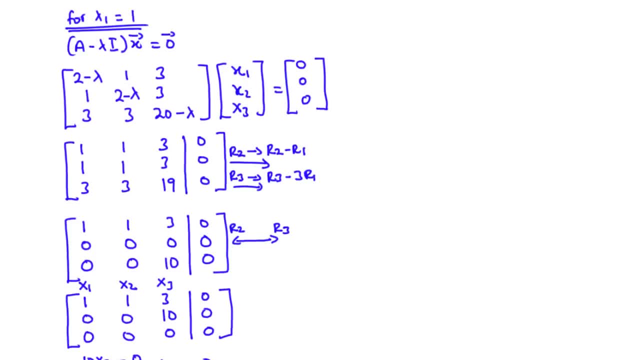 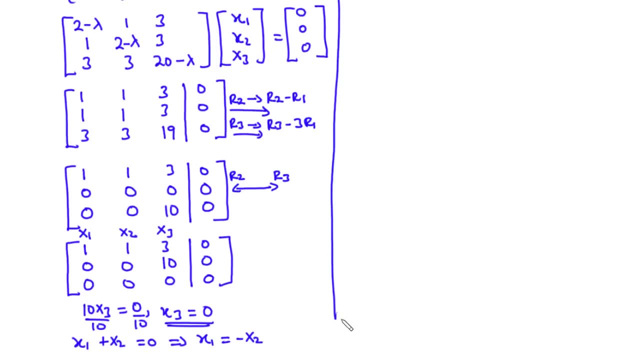 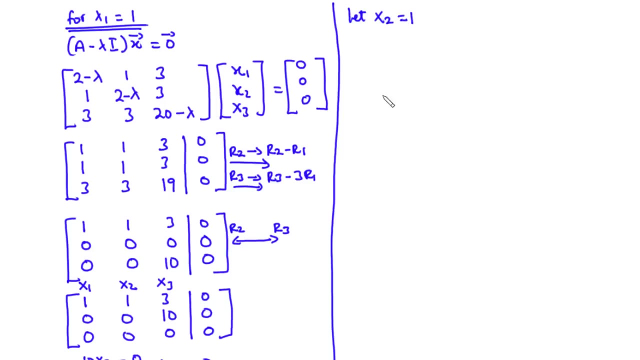 and then at this point, we are going to choose any arbitrary value for x2, so we can say that let x2 equals 1. now, if x2 equals 1, then x1 becomes negative 1, so we have x1 equals negative 1. therefore, the eigenvector x, which has components x1, x2, x3. 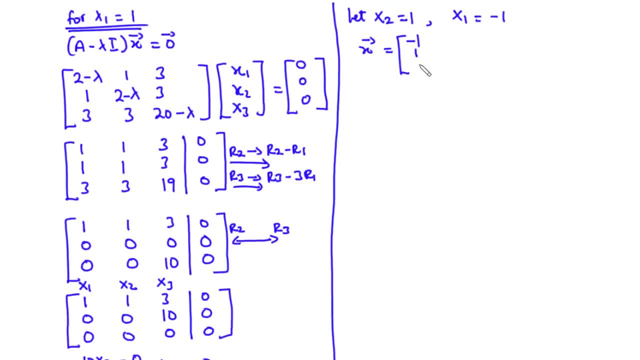 it becomes negative. 1 1: 0 is the eigenvector of A. that corresponds to the eigenvalue lambda1 equals 1.. Now let's move on to the second eigenvalue, that is, for lambda2 equals 2.. Now, if lambda2 is equal to 2 or for lambda2 equals 2, we are going to start from this point. 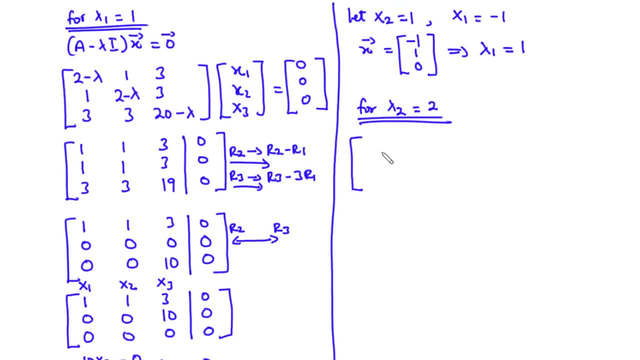 We are going to have 2 minus 2, that is 0,. we have 1, 3,. 1, 2 minus 2 is 0,. we have 3, 3, 3,. 20 minus 2 is 18,. 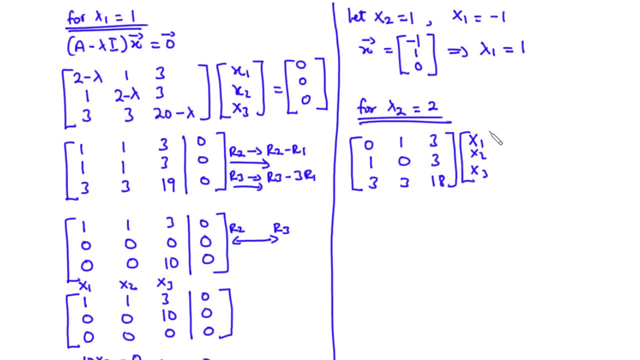 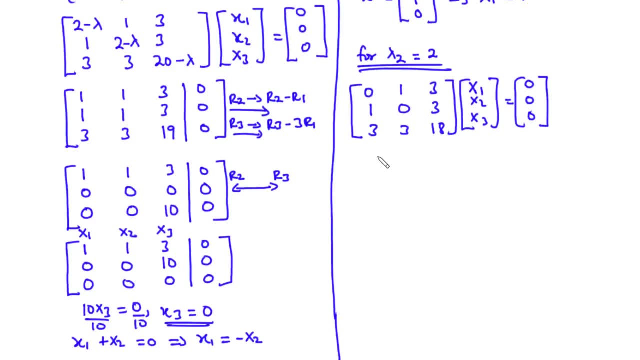 times x1, x2, x3.. Equals 0, 0, 0.. Now let's rewrite this system of equations in the form of augmented matrix. So that is going to be 0, 1, 3, 1, 0, 3, 3, 3, 18.. 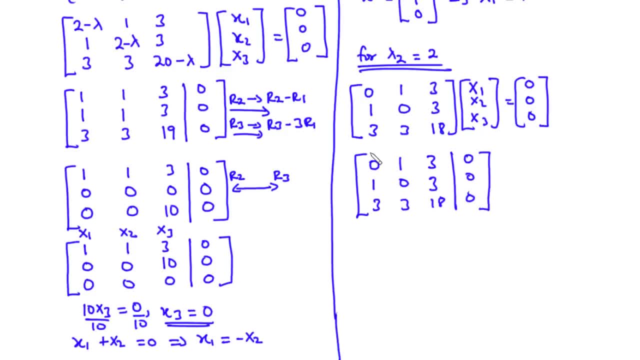 Now, the first thing we are going to do is, because we have a 0 here, we are basically going to interchange row 1 and row 2.. So we interchange row 1 and row 2.. So that we have 1, 0, 3, 0, 0, 1, 3, 0, 3, 3, 18, 0.. 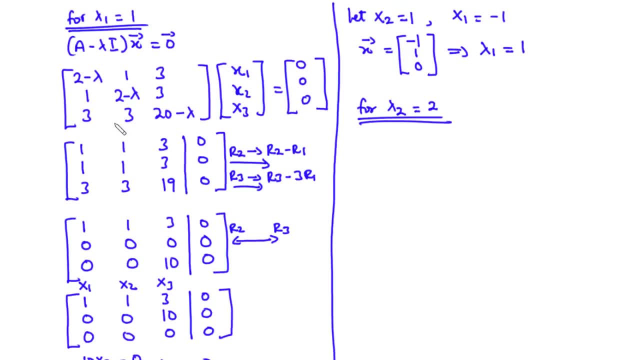 lambda: 2 equals 2. we are going to start from this point. we are going to have 2 minus 2, that is 0. we have 1: 3. 1. 2 minus 2 is 0. we have 3: 3, 3. 20 minus 2 is 18. 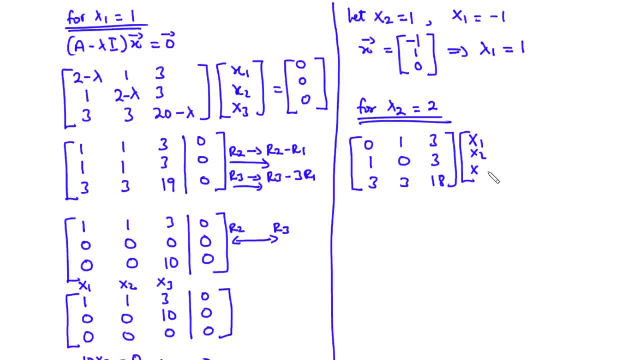 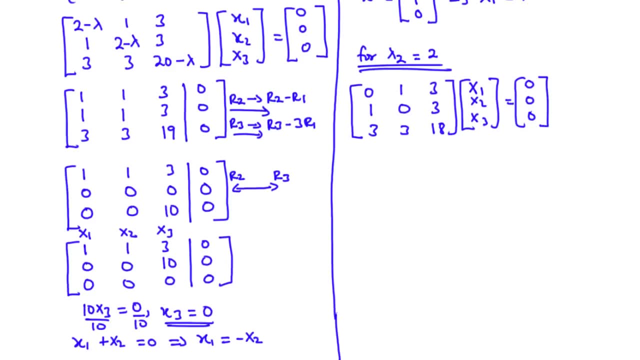 times X, 1, X, 2, X 3 equals 0, 0, 0. now let's rewrite this system of equations in the form of augmented matrix, so that's going to be 0, 1, 3, 1, 0, 3, 3, 3, 18. 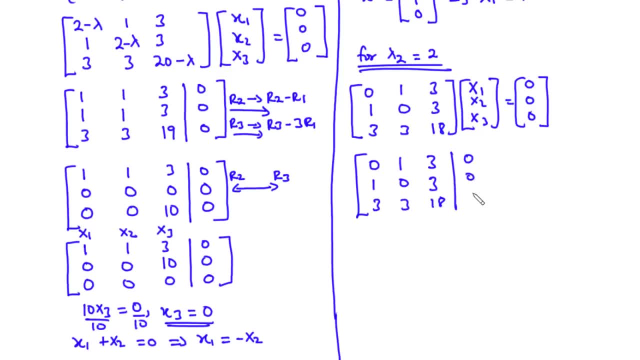 now the first thing we are going to do is, because you have a 0 here, you are basically going to interchange row 1 and row 2, so we interchange row 1, end rule 2, so that we have one zero, three zero, zero. one three zero. 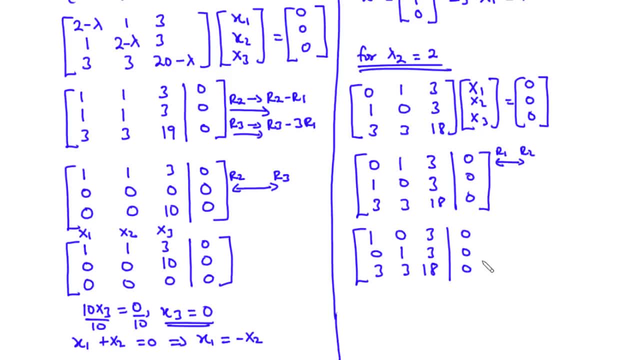 Now this value is already zero, so let's focus on this value. To convert this value to zero, we perform the operation on R3.. And the operation is: we are going to multiply R1 by 3 and subtract that from R3.. 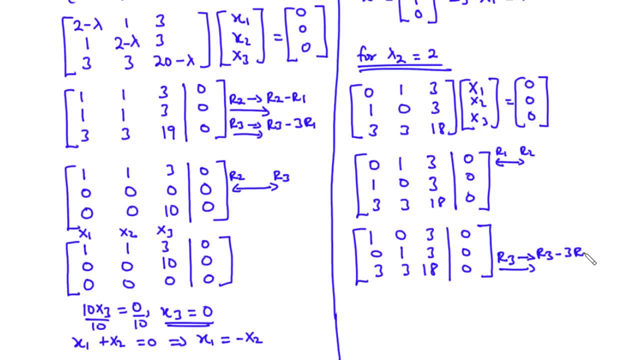 So that is R3 minus 3 times R1.. So this becomes: we have 1, 0, 3, 0, R2 also remains the same, And then for R3, we have 3 minus 3 times 1, that becomes 3 minus 3, that is 0. 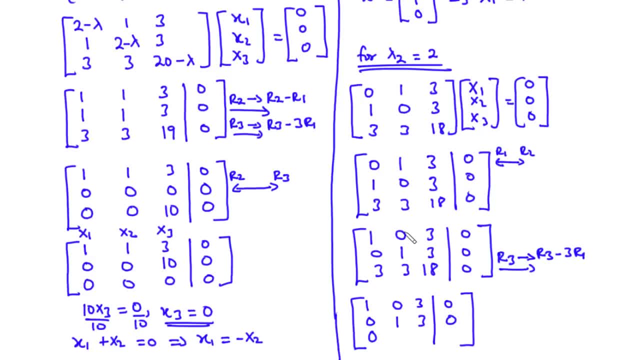 We have 3 minus 3 times 0,. 3 times 0 is 0, so 3 minus 0 is still 3.. And then we have 18 minus 3 times 3.. It's 9.. So 18 minus 9 is 9.. 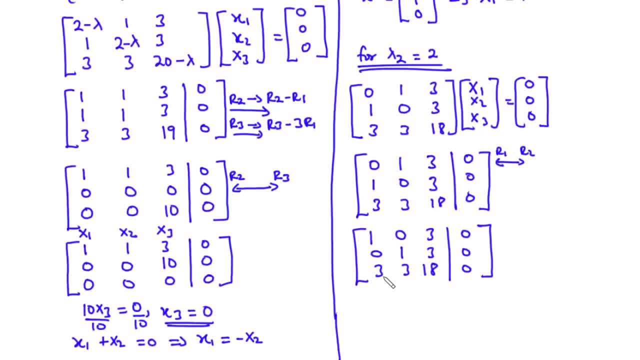 Now this value is already 0, so let's focus on this value. To convert this value to 0,, we perform the operation on R3.. And the operation is: we are going to multiply row 1 by 3 and subtract that from row 3.. 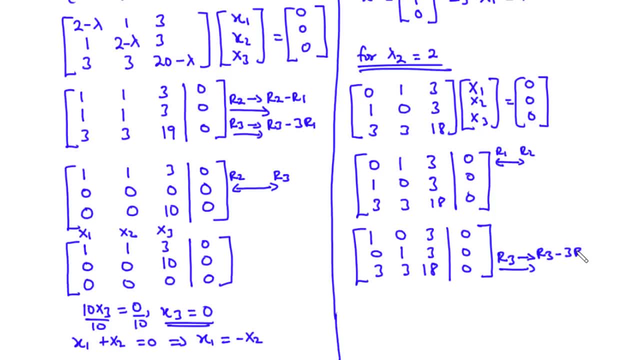 So that is row 3 minus 3 times row 1.. So this becomes: we have 1, 0, 3, 0.. Row 2 also remains the same, And then for row 3, we have 3 minus 3 times 1.. 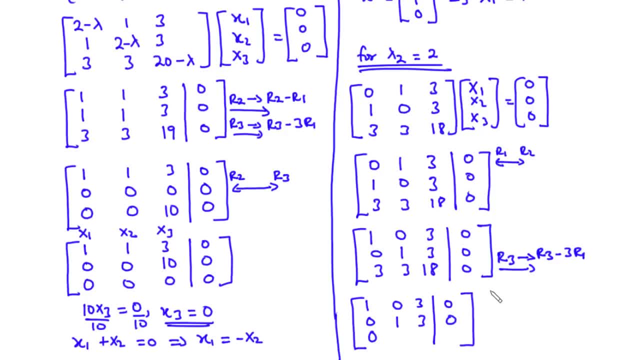 That becomes 3 minus 3.. That is 0.. We have 3 minus 3 times 0.. 3 times 0 is 0.. So 3 minus 0 is still 3.. And then we have 18 minus 3 times 3 is 9.. 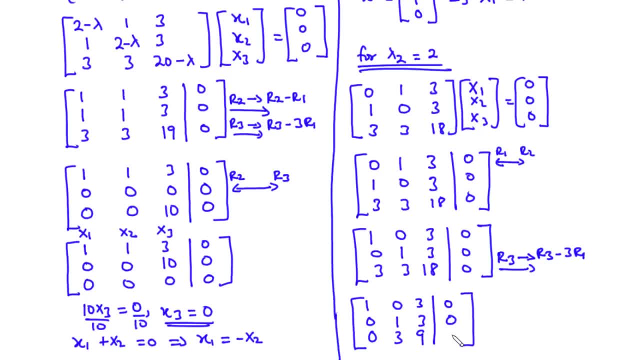 So 18 minus 9 is 9.. And then we have 0 minus 3.. That is still 0.. Now, at this point, we still have this value to be a 3.. Now, to make this value go to 0, we perform the operation on row 3.. 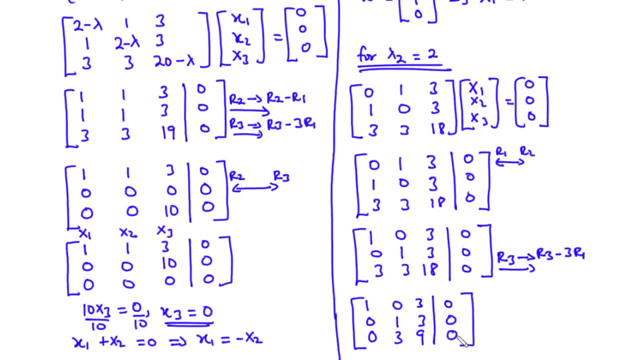 And then we have 0 minus 3 times 0, that is still 0.. Now, at this point, we still have this value to be a 3.. Now to make this value go to 0, we perform the operation on R3.. 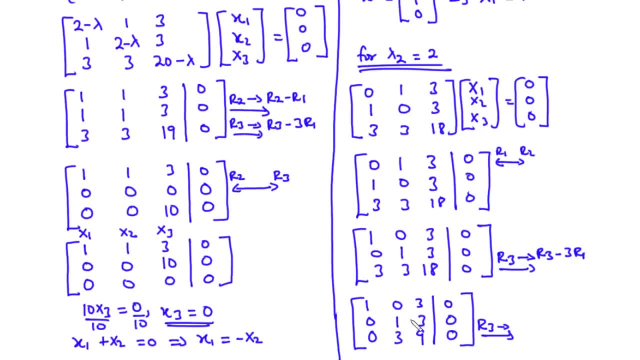 And the operation is: we are going to multiply row 2 by 3 and subtract that from row 3.. So the operation is row 3 minus 3 times row 2. So we have 1, 0, 3.. 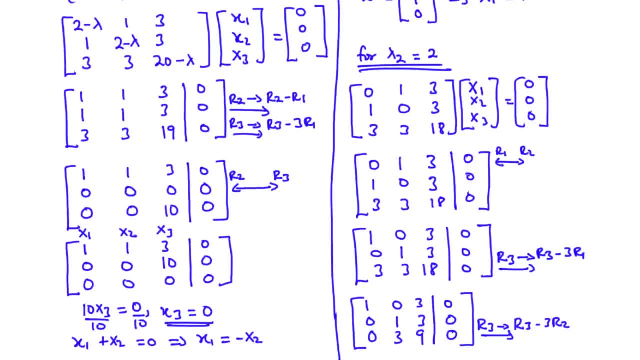 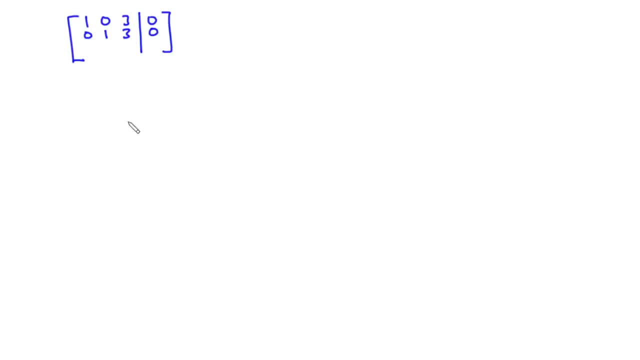 0.. That is for row 1.. For row 2, we have 0, 1, 3, 0.. 0, 1, 3, 0.. And then for row 3, we have 0 minus 3 times 0.. 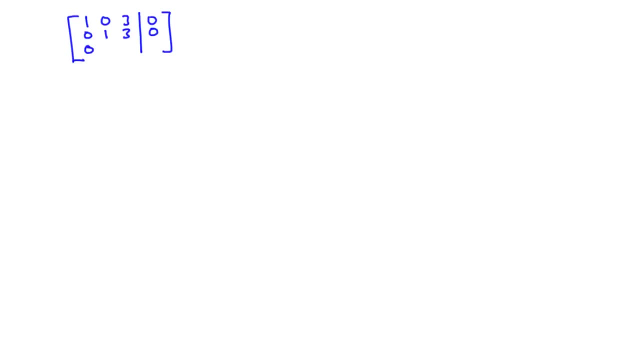 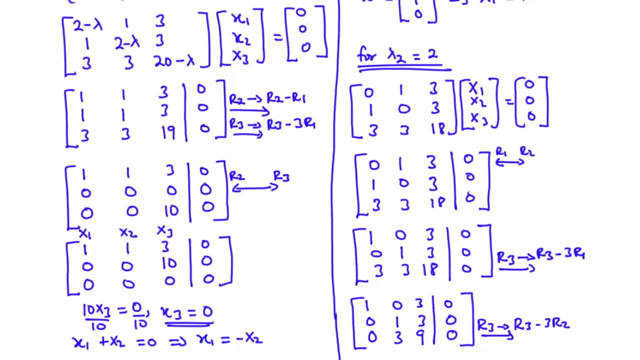 And that is still 0.. We have 3 minus 3 times 1., And that is 3 minus 3.. That is also 0.. We have 3 minus 3 times 1. And that is 3 minus 3.. 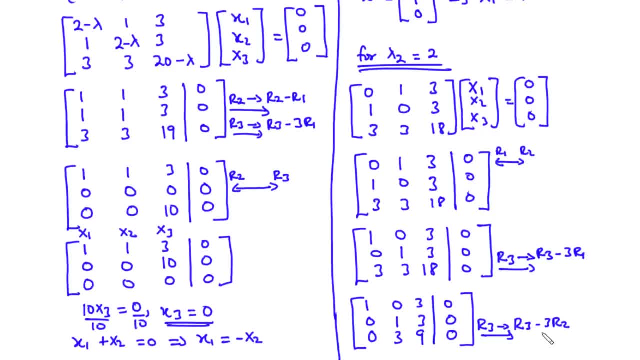 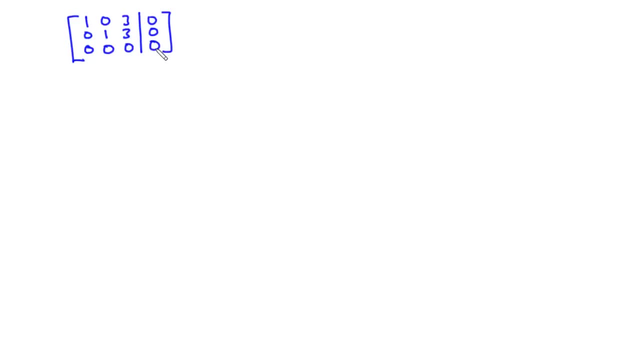 That is also 0. And then we have 9 minus 3 times 3,, which is also 9.. Therefore, 9 minus 9 is 0.. And then 0 minus 3 times 0 is still 0.. So we have 0 here and then 0 here. 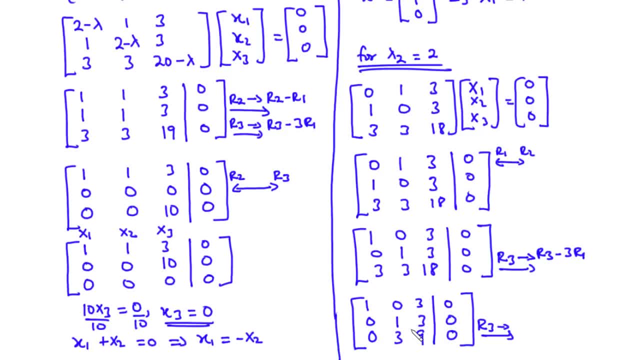 And the operation is: we are going to multiply R2 by 3 and subtract that from R3.. So the operation is R3 minus 3 times R2.. So that is R3 minus 3 times R2.. So that is R3 minus 3 times R2.. 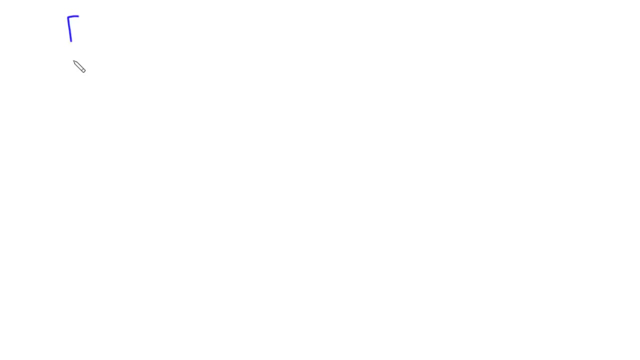 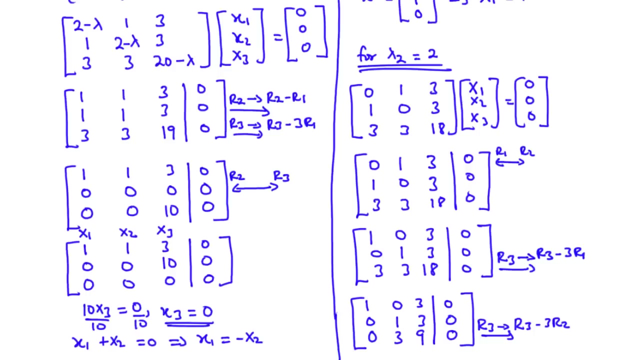 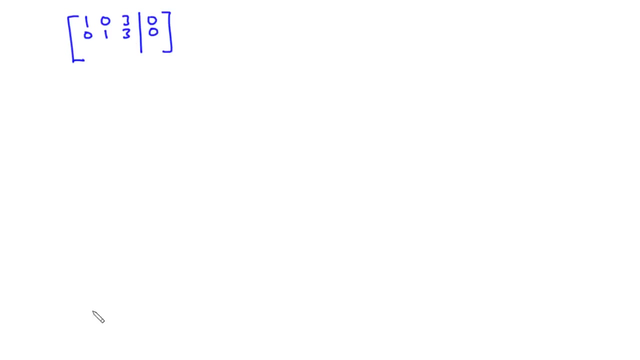 So that is R3 minus 3 times R2.. So we have 1, 0, 3, 0,. that is for R1, for R2 we have 0, 1, 3, 0, 0, 1, 3, 0. 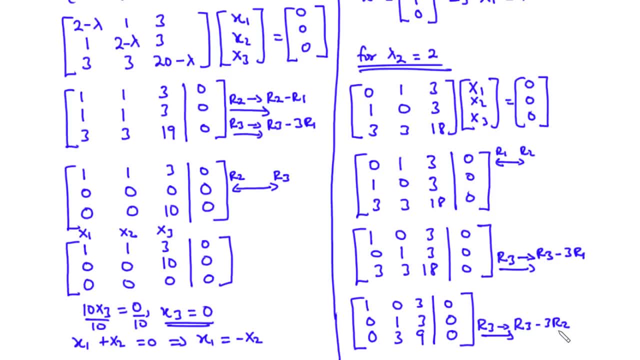 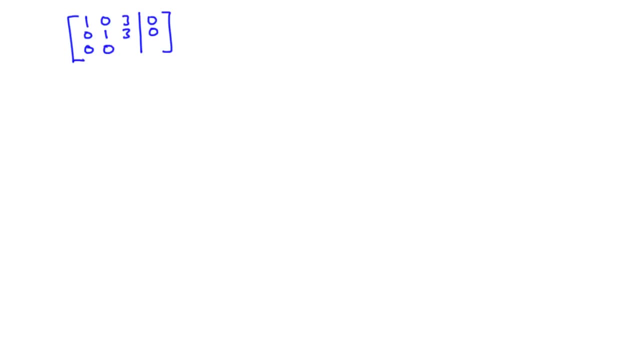 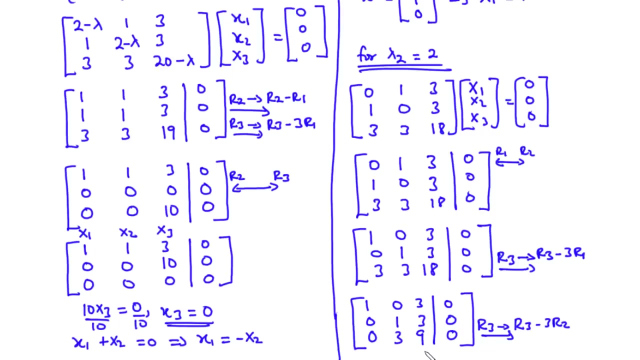 And then for R3, we have 0 minus 3 times 0,, and that is still 0. We have 3 minus 3 times 1. And that is 3 minus 3.. That is also 0. And then we have 9 minus 3 times 3,, which is also 9.. 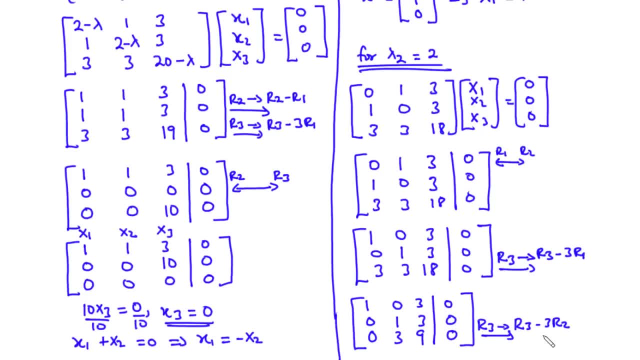 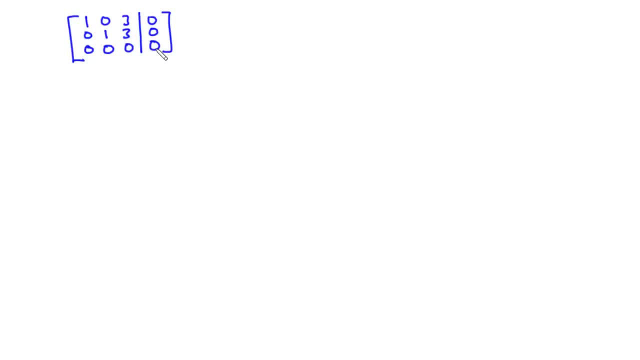 Therefore, 9 minus 9 is 0.. And then 0 minus 3 times 0 is still 0.. So we have 0 here and then 0 here. So this is the row echelon form of the augmented matrix. Now let's focus on R2.. 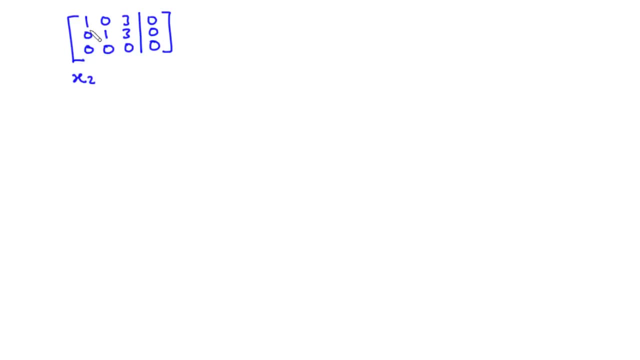 So from row 2, we have x2, x2 plus 3x3 equals 0.. So let's transpose 3x3 to the right hand side And then we have x2 equals negative 3x3.. Now let's choose any arbitrary value for x3.. 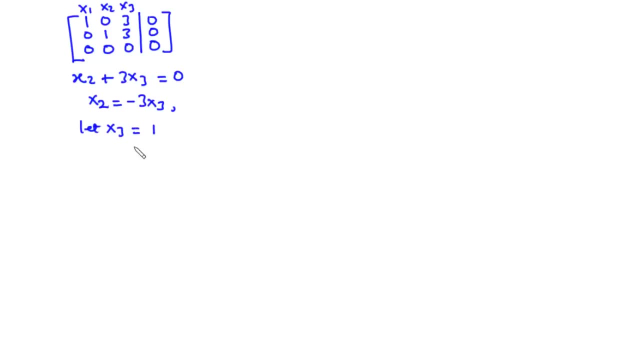 So let's: x3 equals negative 3x3.. Now let's choose any arbitrary value for x3.. Now, if x3 equals 1, then we have x2 to be equal to negative 3 times 1,, which is equal to negative 3.. 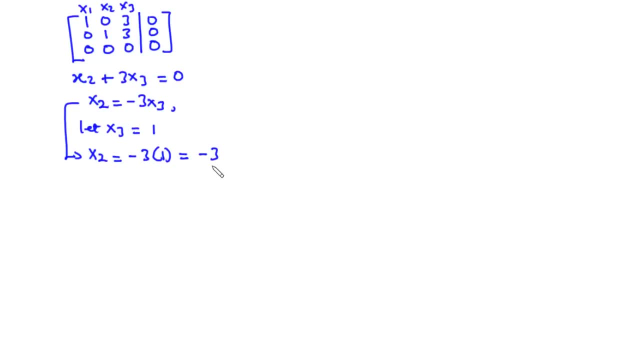 So we have x3 to be 1 and then x2 to be negative, 3.. Now let's focus on row 1.. So for row 1, we have x1 plus 0x2 plus 3x3.. So we have x1 plus 0x2 plus 3x3 equals 0.. 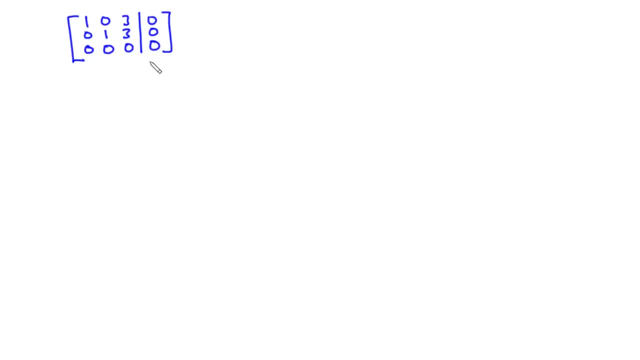 So this is the row echelon form of the augmented matrix. Now let's focus on row 2.. So from row 2, we have x2.. x2.. x2., x2., x2., x2., x2.. 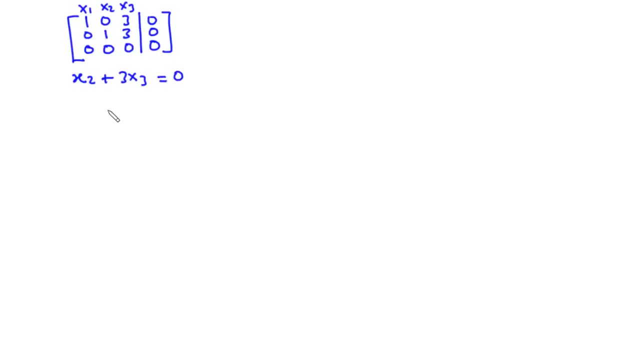 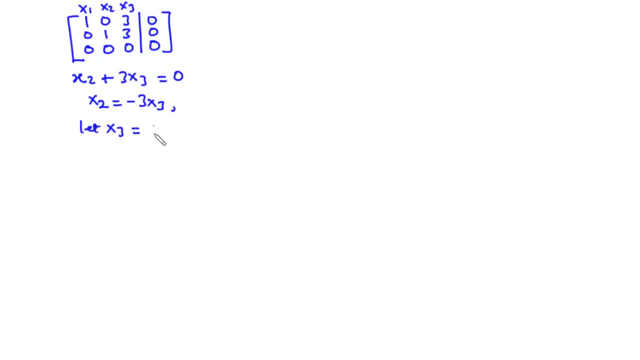 Now let's transpose 3x3 to the right hand side And then we have: x2 equals negative 3x3.. Now let's choose any arbitrary value for x3.. So let's say x3 equals 1.. Now if x3 equals 1.. 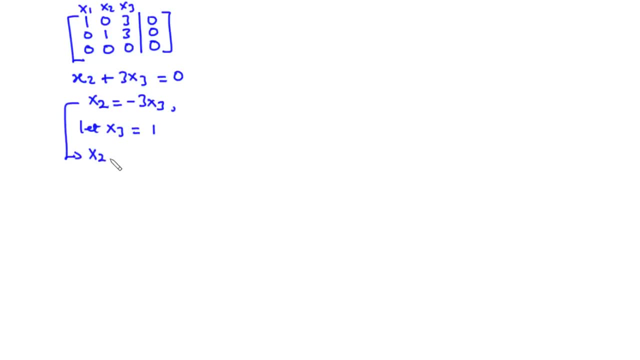 Then we have x2 to be negative 3x3.. Now, if x3 equals 1.. Then we have x2 to be negative 3x3.. to be equal to negative 3 times 1, which is equal to negative 3.. So we have x3 to be 1 and then x2. 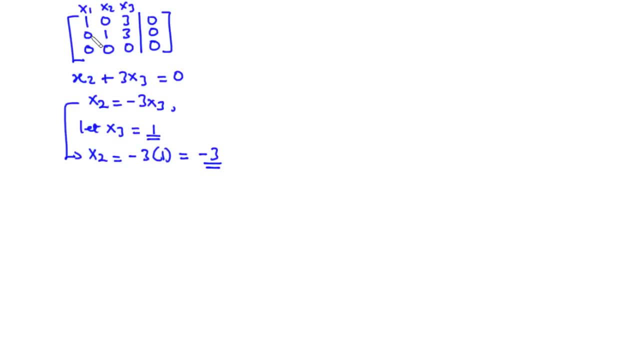 to be negative 3.. Now let's focus on row 1.. So for row 1 we have x1 plus 0x2 plus 3x3 equals 0.. Therefore we have x1 plus 3 times x3 is 1.. So x1 equals negative 3. Therefore, 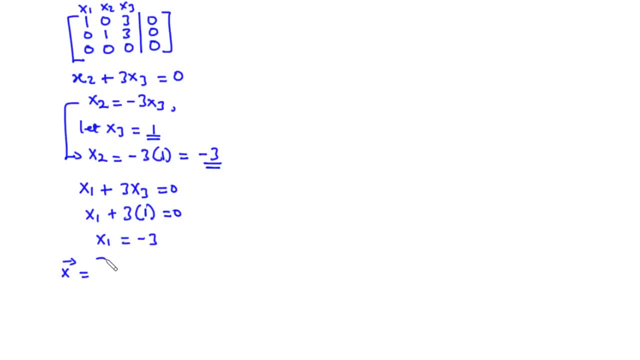 we have the eigenvector x equals negative 3, negative 3, 1, and that is the eigenvector that corresponds to x1.. That corresponds to lambda 2, equals 2.. So now let's find the eigenvector that corresponds. 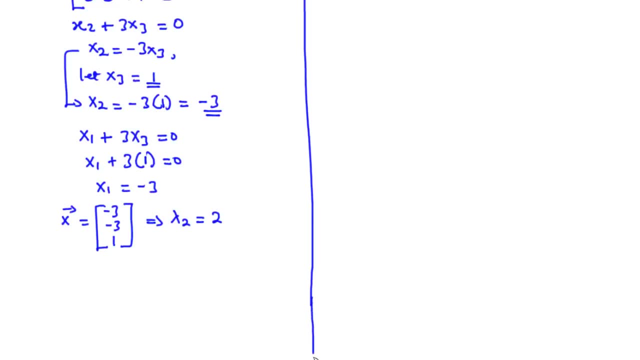 to the last eigenvalue, that is, lambda 3 equals 21.. So for lambda 3 equals 21,. we have 2 minus lambda, So for lambda 3 equals 21.. So 2 minus lambda equals 2 and lambda 3 equals 2.. So for last, 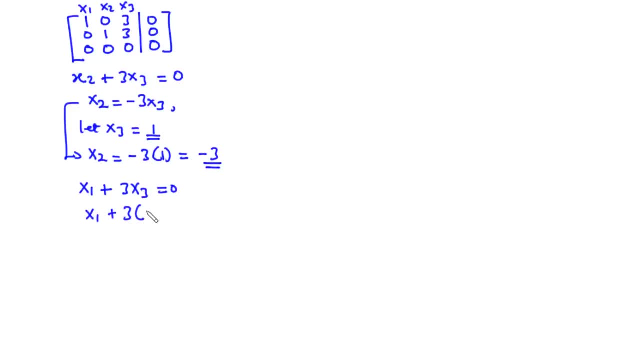 Therefore we have x1 plus 3 times x3 is 1. So x1 equals negative 3. Therefore we have the eigenvector x equals negative 3, negative 3, 1. And that is the eigenvector x. 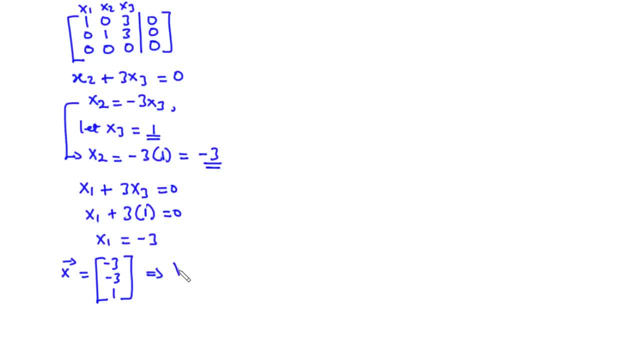 And that is the eigenvector x. And that is the eigenvector x that corresponds to lambda 2 equals 2. so now let's find the eigenvector that corresponds to the last eigenvalue, that is lambda 3 equals 21. so for lambda 3, 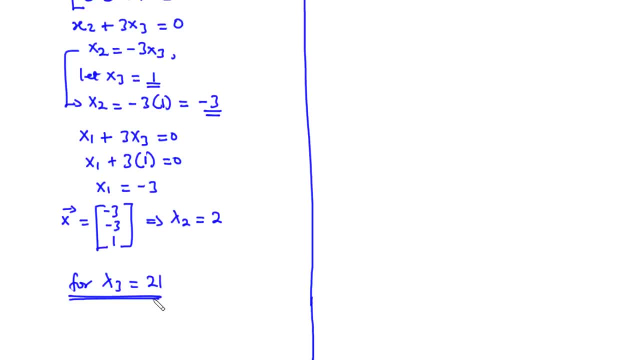 equals 21. we have 2 minus lambda 1, 3, 1, 2 minus lambda 3, 3, 3, 20 minus lambda times x1, x2, x3 equals 0, 0, 0. so in place of lambda, we have lambda 3, which is 21, so that's going to be 2. 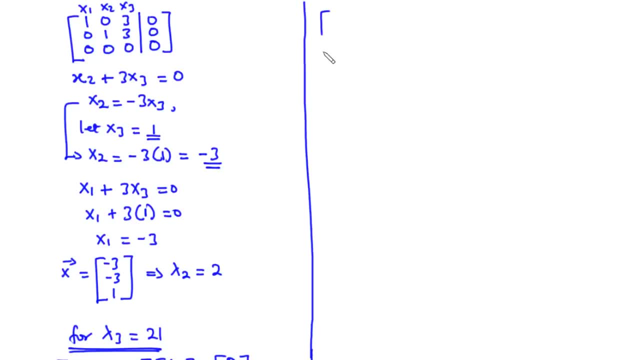 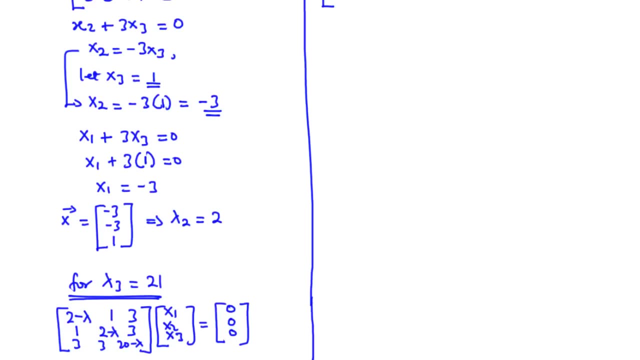 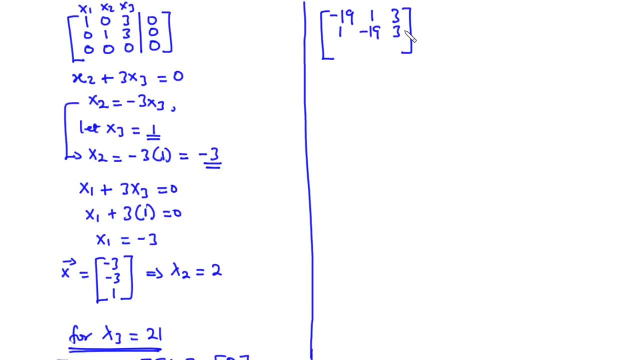 minus 21, that is negative 19. so we have negative 19, negative 19. one, three one, and then 2 minus 21 is negative 19. 3, 3, 3 and then 20 minus 21 is negative 1. so we have this times X, 1, X, 2, X, 3. all equals 0, 0, 0. now let's rewrite the. 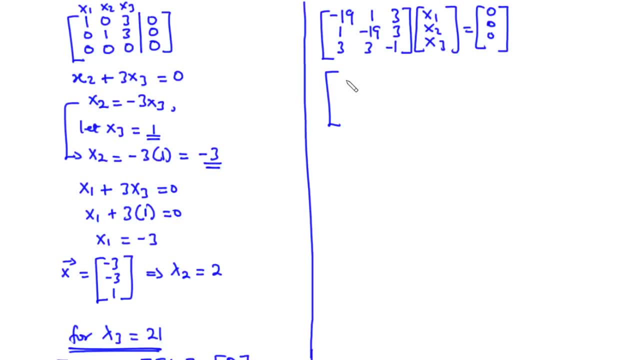 system of equations in an augmented matrix. so we have negative 19, 1, 3 1. negative 19, 3, 3, 3. negative 1, 0, 0, 0. now to make these values go to 0, we perform the operation on row 2 and the operation is: we are going to multiply row 2. 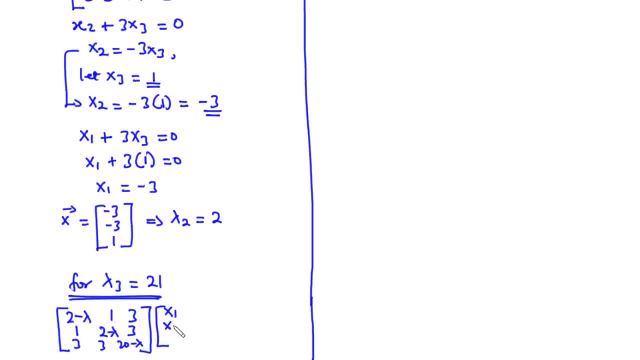 eigenvector x equals 2 minus dre more than 2.. So x2 plus 2 plus lambda equals 2.. Why is this break Volks reading? Пока La Tr deste Landscape. So we have in place of lambda here we have lambda3 and we have lambdaNного. So we have lambdaN RefresovenL's besten scheme, that is plug in that we have in place of laughdata. So now we have lambdaDish. We have 3 of lambdaDish. We already know that lambda2 is 21.. And now? 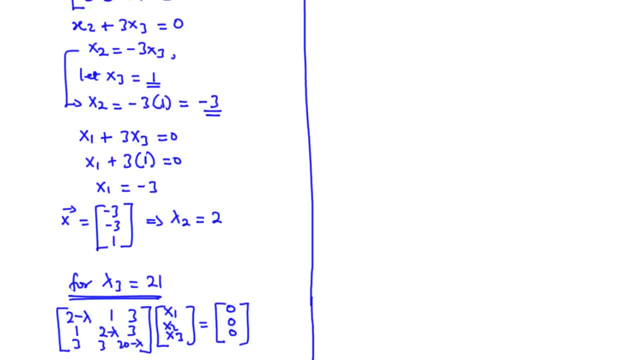 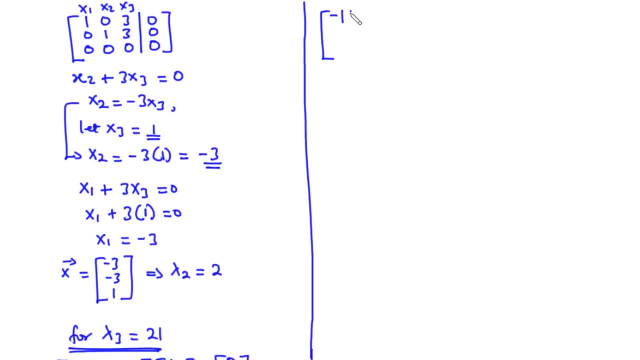 we have x1 plus 1x2x3.. And for lambda3.. So this will be negative 35. California indexed American- And who did that? minus 21,. that is negative 19,. so we have negative 19,. negative 19,. 1,, 3,, 1, and then 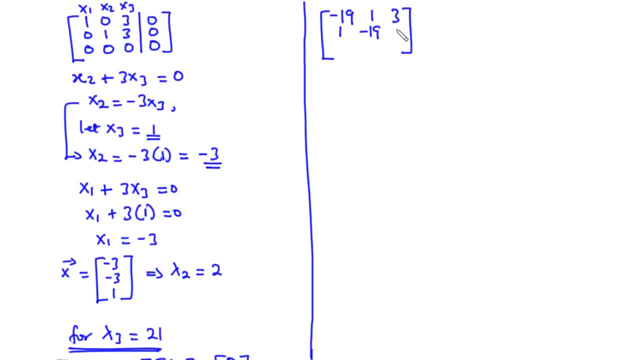 2 minus 21 is negative 19,, 3,, 3,, 3, and then 20 minus 21 is negative 1, so we have this times: x1, x2, x3, all equals 0, 0, 0,. now let's rewrite the system of equations. 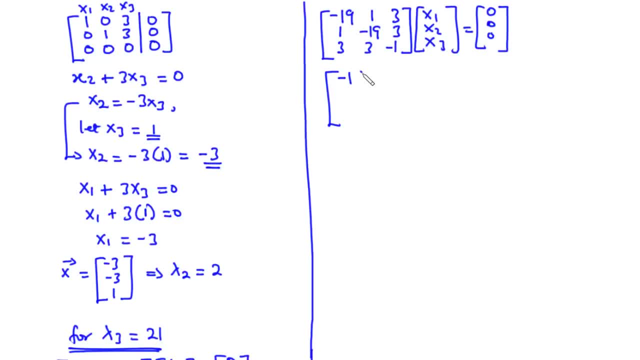 in an augmented matrix. so we have negative 19, 1, 3, 1, negative 19, 3, 3, 3, negative 1, 0, 0, 0,. now to make these values go to 0, we perform the operation on row 2, and. 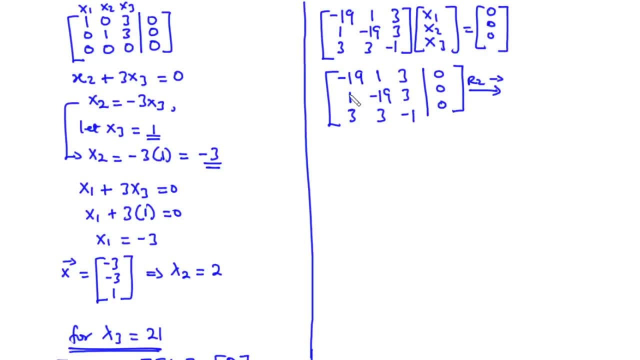 the operation is: we are going to multiply row 2 by 30.. We are going to subtract that from row 3, so row 3 minus 3 times row 2, and also for row 3, we are going to use the same operation, that is, we multiply row 2 by 3 and subtract. 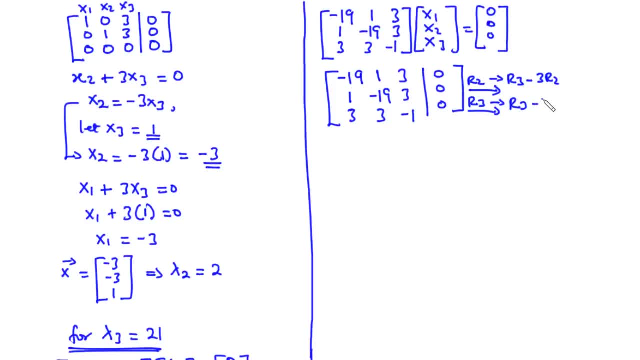 that from row 3, so we have r3 minus 3r2,, so element in row 1 remains the same. and then for row 2, we have 3 minus 3 times 1, which is 0,, 3 minus 3 times negative 19.. 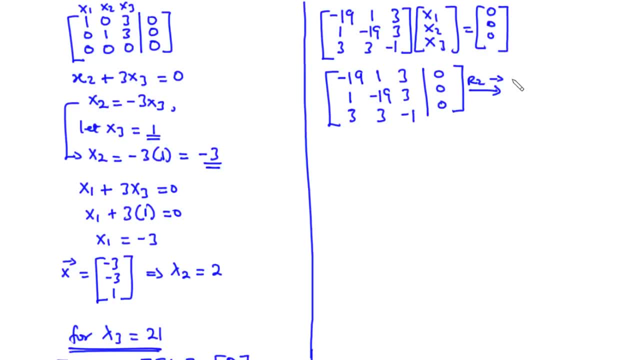 by 3 and subtract that from row 3, so row 3 minus 3 times row 2. and also for row 3 we are going to use the same operation, that is, we multiply row 2 by 3 and subtract that from row 3, so we have R 3 minus 3 R 2, so element in row 1 remains. 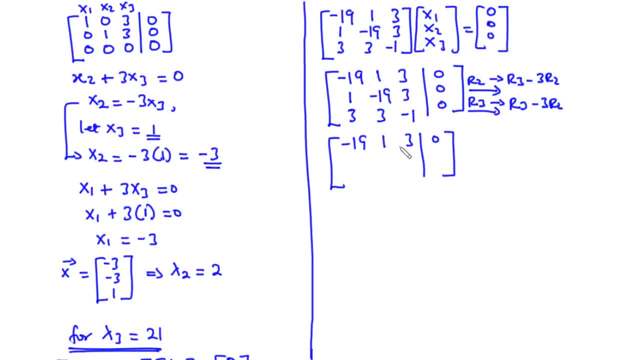 the same. and then for row 2 we have 3 minus 3 times one, which is 0, 3 minus 3 times negative 19, now negative 3 times negative. 19 is 57. so 3 plus 57 is 60 negative. 1 minus 3 times 3 is negative. 1 minus 9 and that is negative 2.. kicking. 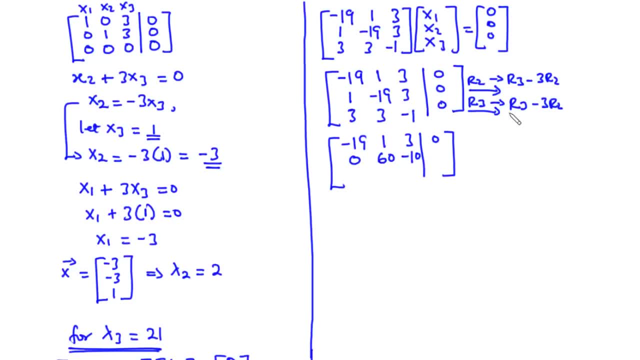 negative 3 times negative 2. that is inside that. so negative 3 minus 3 times 3 is negative 50alted. so we're going to multiply and that is negative 10, and then 0 minus 3 times 0 is still 0. now we still have the same thing here. 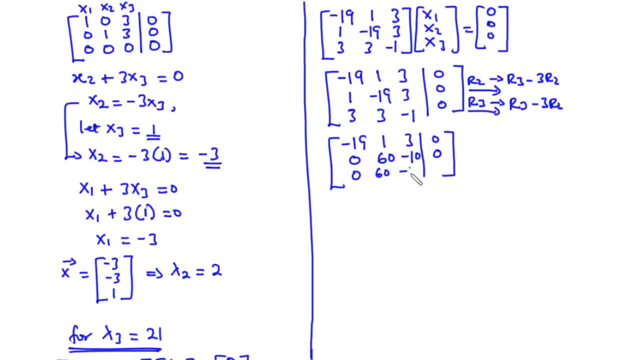 so we are going to have 0, 60 negative 10: 0.. now let's try to make this value go to 0. so we perform the operation on row 3, and the operation is: we are going to subtract row 3 from row 2, so that is row 2 minus row 3, and then we have negative 19, 1, 3, 0. 60 negative 10. 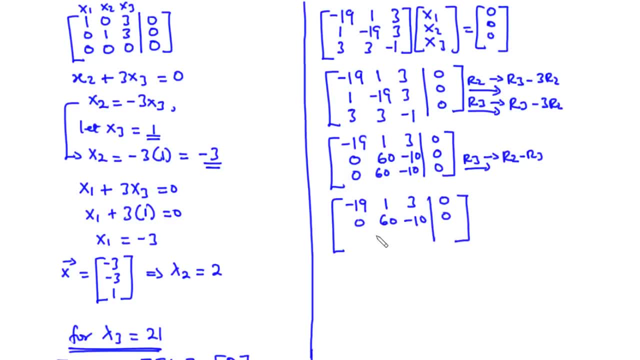 0- 0. for row 3 we have: 0 minus 0 is 0, 60 minus 60 is 0. negative 10 minus negative 10 is still 0, and then 0 minus 0 is also 0, because we want to make this value 1 and also this value 1. 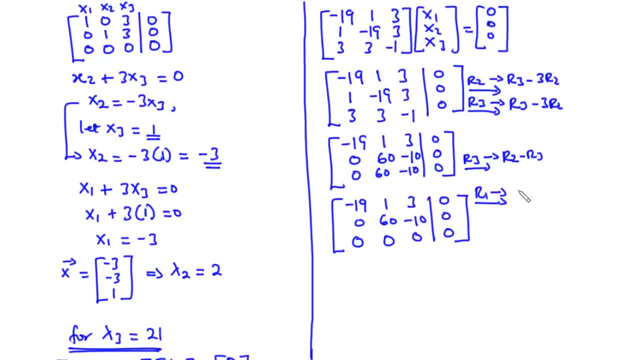 we perform operation on row 1, and that's: we multiply negative 1 over 19 by row 1. also for row 2, we multiply 1 over 60 by r2. so let's do that now we have negative 19 times negative 1 over 19. 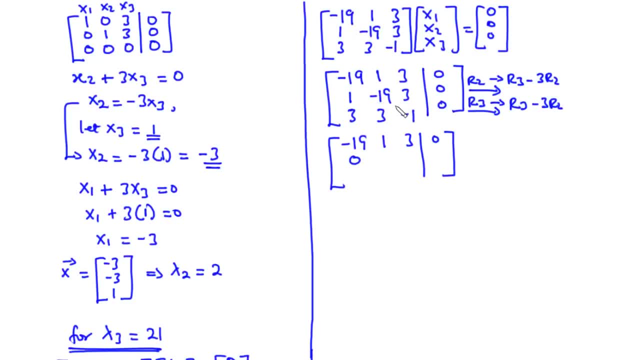 Now negative 3 times negative. 19 is 57, so 3 plus 57 is 60, negative 1 minus 3 times 3 is negative 1 minus 9, and that is negative 10.. Thank you for watching. 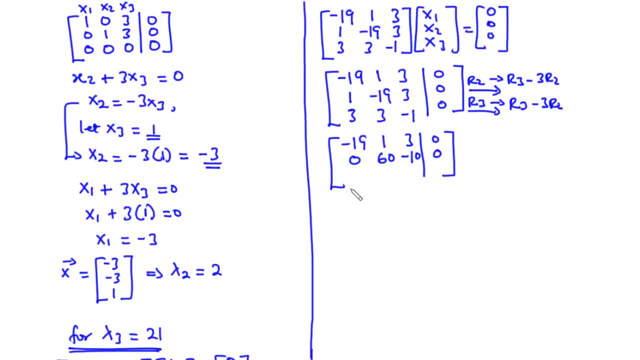 And then 0 minus 3 times 0 is still 0.. Now we still have the same thing here. So we are going to have 0, 60, negative 10, 0.. Now let's try to make this value go to 0. 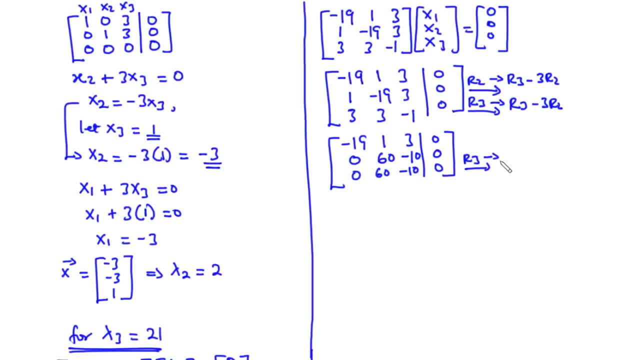 So we perform the operation on row 3.. And the operation is: we are going to subtract row 3 from row 2.. So that is row 2 minus row 3.. And then we have negative 19,, 1, 3, 0, 60,. negative 10, 0, 0.. 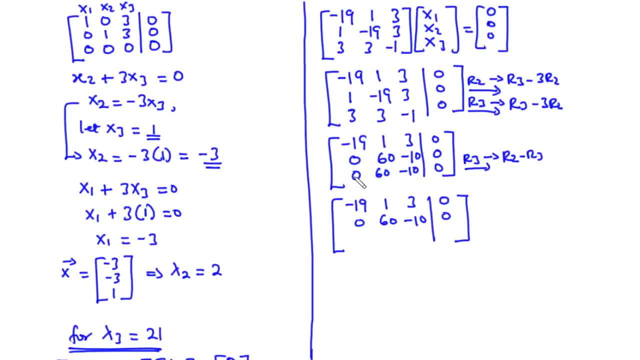 For row 3, we have: 0 minus 0 is 0.. 60 minus 60 is 0.. Negative 10 minus negative 10 is still 0. And then 0 minus 0 is also 0. Because we want to make this value 1 and also this value 1,. 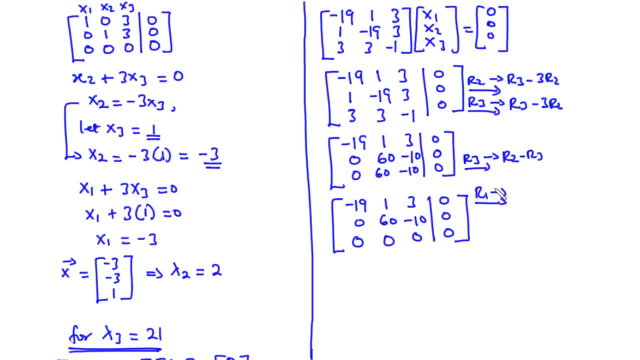 we perform operation on row 1.. And thus we multiply negative 1 over 19 by row 1.. Also for row 2, we multiply 1 over 60 by row 2.. So let's do that Now we have negative 19 times negative 1 over 19.. 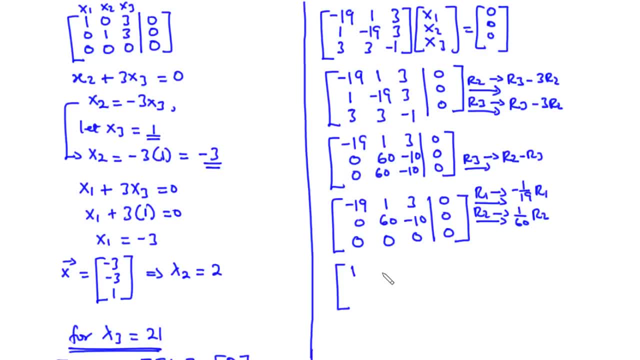 That is 1.. 1 times negative: 1 over 19.. That is negative. 1 over 19.. 3 times negative: 1 over 19 is negative. 3 over 19.. And then 0 times. anything else here is still 0.. 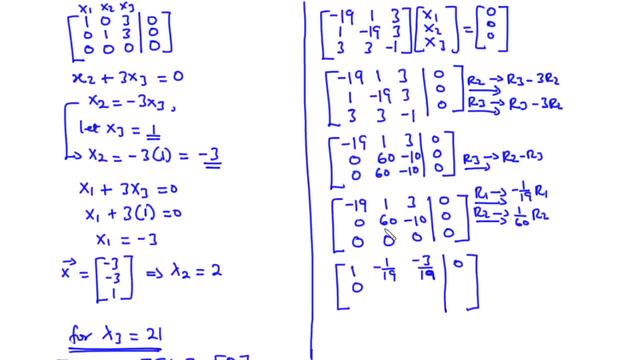 For row 2, we have 1 over 60 times 0.. That is 0.. 1 over 60 times 60 is 1.. 1 over 60 times negative. 10 is negative. 1 over 6.. And then 0 times anything here is still 0.. 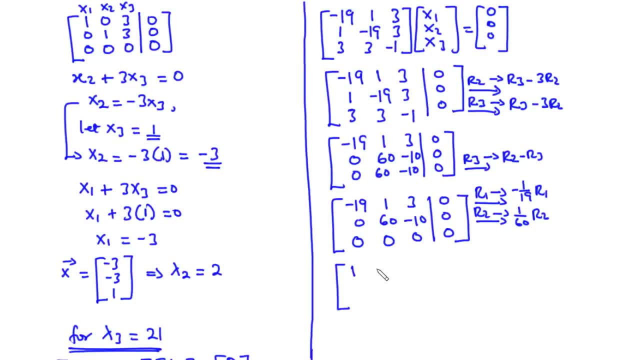 that is 1, 1 times negative. 1 over 19, that is negative. 1 over 19,. 3 times negative: 1 over 19 is negative. 3 over 19 and then 0 times. anything else here is still 0.. 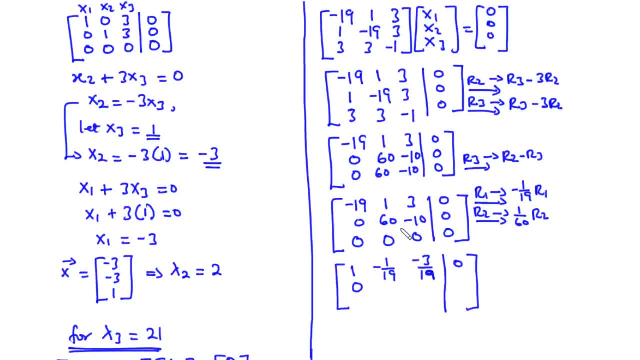 For row 2 we have 1 over 60 times 0, that is, 0,. 1 over 60 times 60 is 1, 1 over 60 times negative. 10 is negative. 1 over 6 and then 0 times. anything here is still 0 and then. 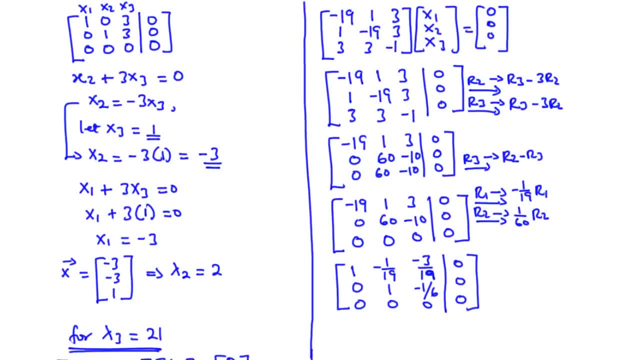 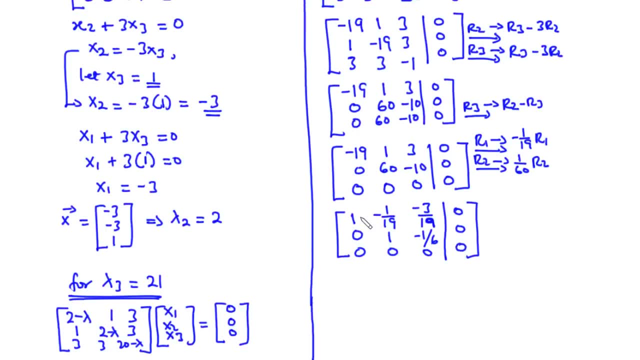 we have 0, 0, 0, 0.. Now, at this point, let's focus on row 2.. So for row 2, we have x2, we have x2 minus 1 over 6 x3. We can simplify this as x2 equals 1 over 6 x3 and we say that let x3 be equal to 1.. 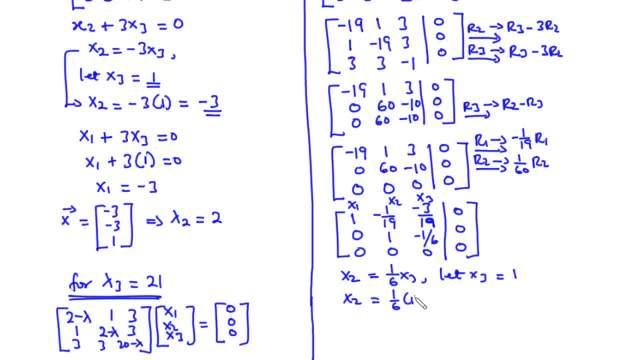 In that case we have x2 equals 1 over 6 times 1, which is still 1 over 6.. So we have x3 equals 1, x2 equals 1 over 6.. Now to find the value of x3 and x2 equals 1, we have x2 equals 1 over 6 and x2 equals. 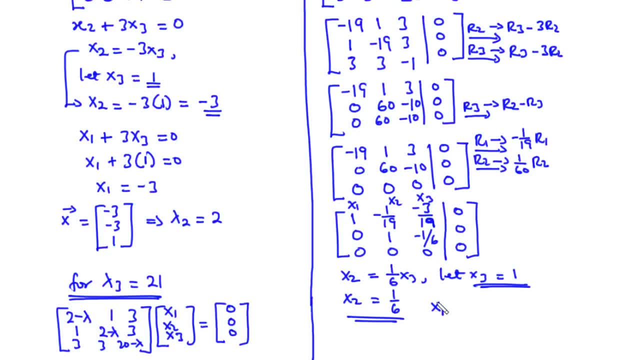 value of x1, we have x1 equals 1 over 19 x2, plus 1 over- sorry, we have 3 over 19 x3. Now x2 is equal to 1 over 6 and then x3 is 1.. 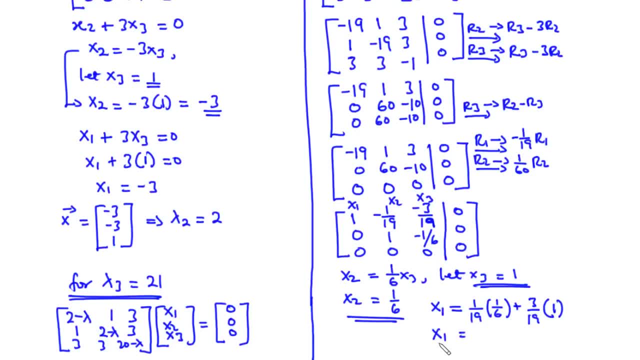 So if you add these two fractions, you are going to get x1 to be equal to 1 over 6.. Therefore, the eigenvector x, which has components 1 over 6,, 1 over 6,, 1. Is the x1.. 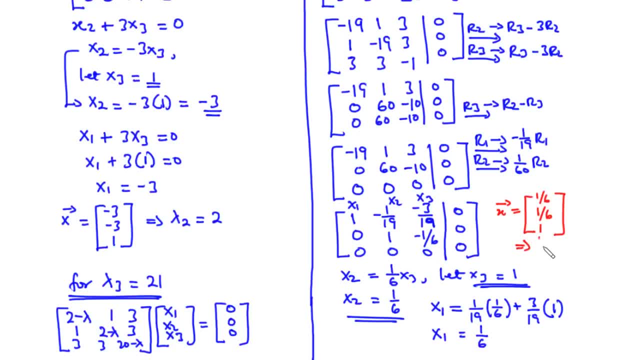 The eigenvector that corresponds to lambda 3 equals 21..